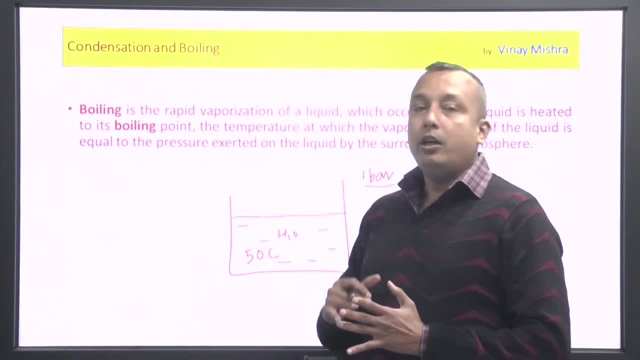 is that we know that water boils at 100 degree centigrade. that means the liquid phase changes, because boiling is a process by which the phase transformation takes place from liquid to vapor form. that means when liquid changes in vapor form, then this process is called. 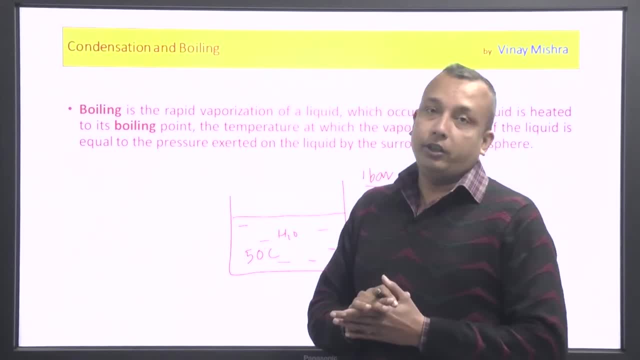 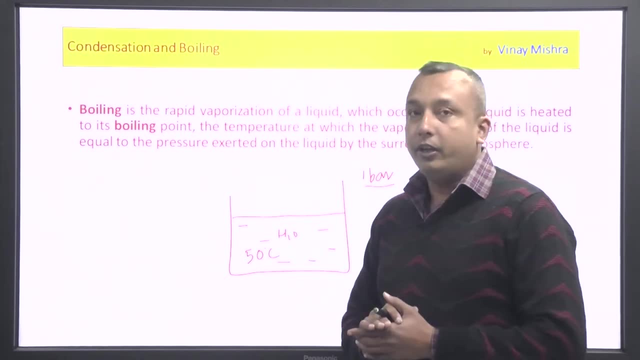 basically boiling, and this happens when our temperature exceeds at a certain point. For example, we assume that the initial temperature is 50 degree centigrade. In general, we assume that 100 degree centigrade is the boiling temperature, but this is not. 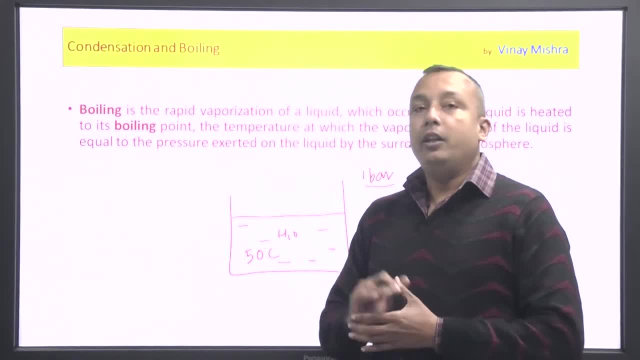 correct at all times, because it is not necessary to boil water at 100 degree centigrade. water can be at less than 100 degree centigrade or at more than 100 degree centigrade. this will depend on you. Basically, the temperature at which the temperature exceeds is called boiling. 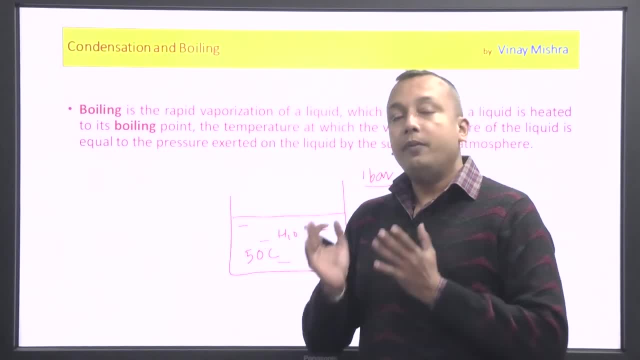 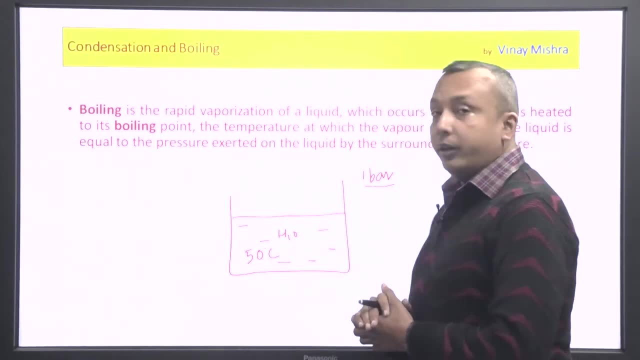 So atmospheric pressure is how much? because the vapor pressure corresponding to it will be valid. So here, if we talk about 50 degree, centigrade is the initial temperature of water. atmospheric pressure is 1 bar. The corresponding saturation temperature of 1 bar is basically approximately 100 degree. 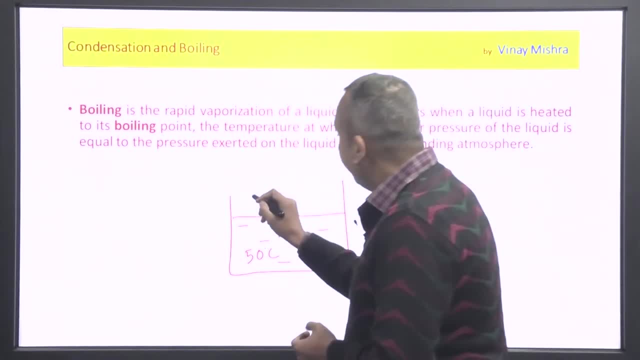 centigrade. What happens basically? if we understand boiling a little more deeply, then atmospheric pressure is according to this same. If we compare it exactly at 0 degree centigrade, then it may be liable that there will be 180 degree centigrade period of automatic pressure. 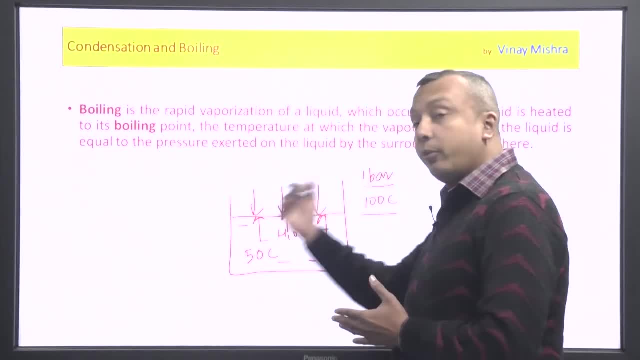 This is for agglutination of liquid. That is for agglutination of required liquid. How much radiation Porkorite does Take 80 kg and feed it for 10 kg of press directly to the one Australia that is for. 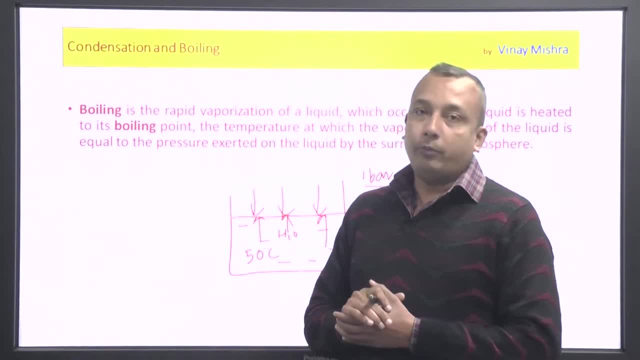 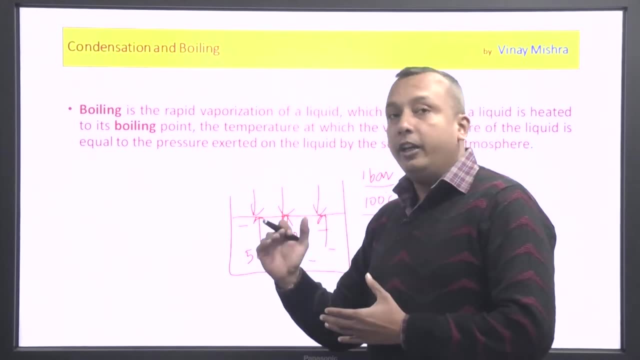 wspóling. So this will be log dipole. Wapor pressure is approximately 5 degree centigrade Come thisOC in half unquote means about 50 degree centigrade. happens here in this case, where it has 70 degree centigrade pressure covered up at 90 degree centigrade the temperature. 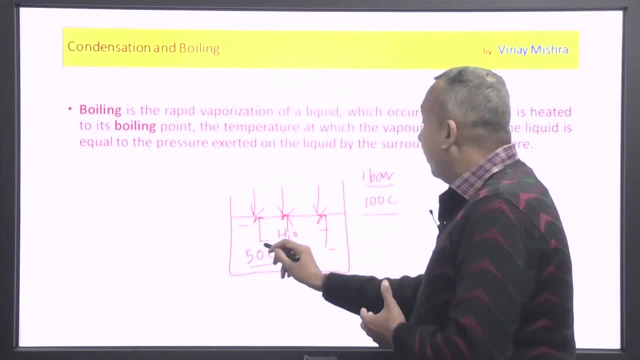 after which Esp lie. So that still remains 1 bar, or say, in case of a mean days, e $1.. So now notice, up to something like 700 degree centigrade, Isn't there, will be equal to the corresponding saturation temperature. then we will say that a condition. 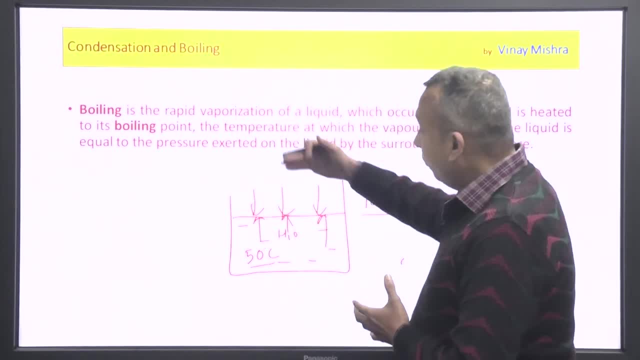 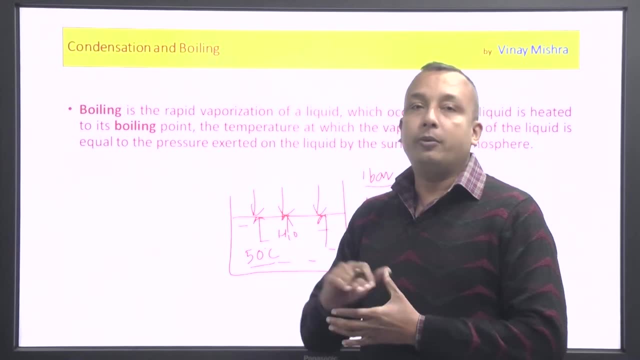 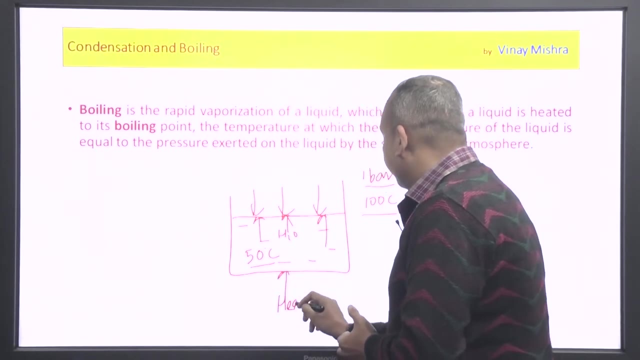 will come here, in which the water molecules will start escaping there. basically that process will happen of boiling, or we will say of vaporization, in which the phase transformation will start happening here. so for example, here we are giving heat as soon as we give. 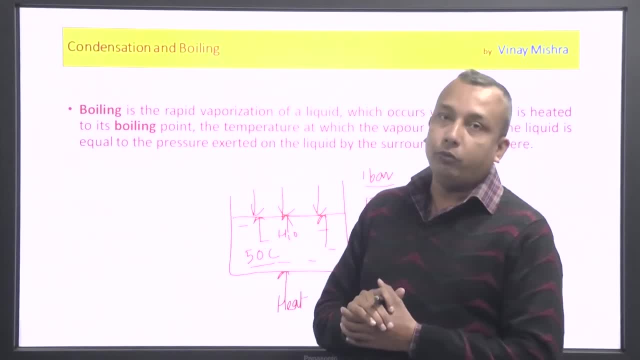 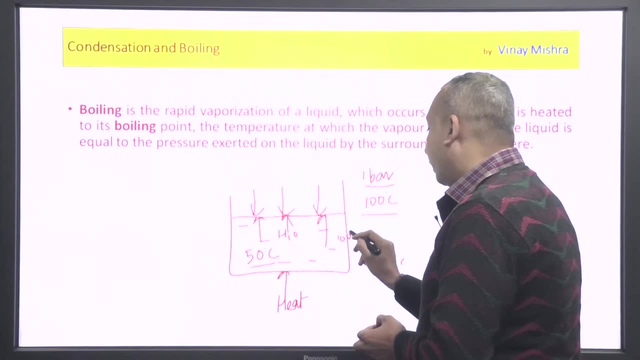 heat, its temperature will rise. the boiling will not happen at 50 degree centigrade. at 50 degree centigrade, the boiling will not start. when the boiling will not start till, its temperature will not become 100 degree centigrade. as soon as its temperature will. 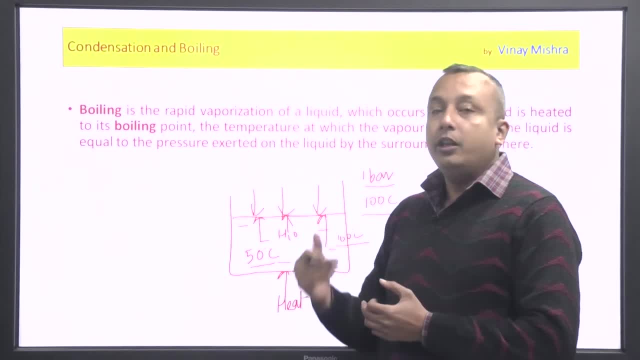 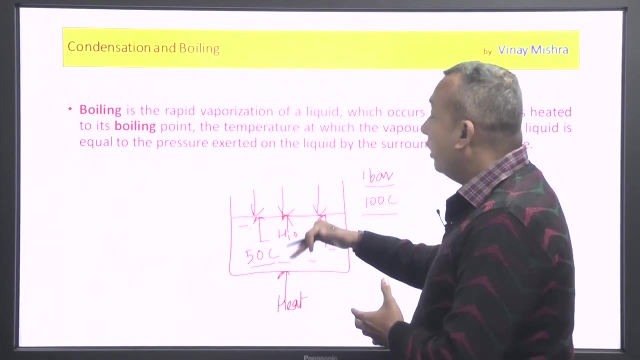 keep increasing 51,, 60,, 70,, 80,, 90, till approximately at 100 degree centigrade. here what will happen? these molecules will have sufficient energy and they will escape this liquid surface. now, here, transformation will start here. liquid, liquid, liquid, the liquid, the liquid. 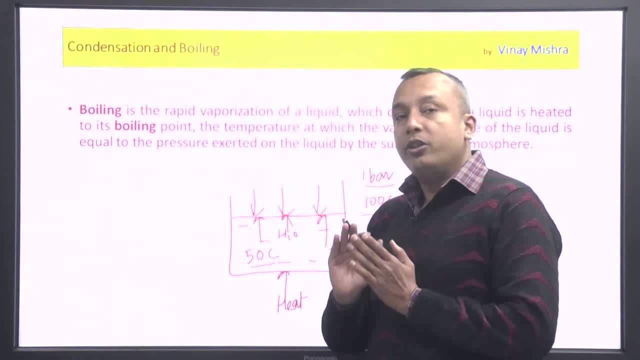 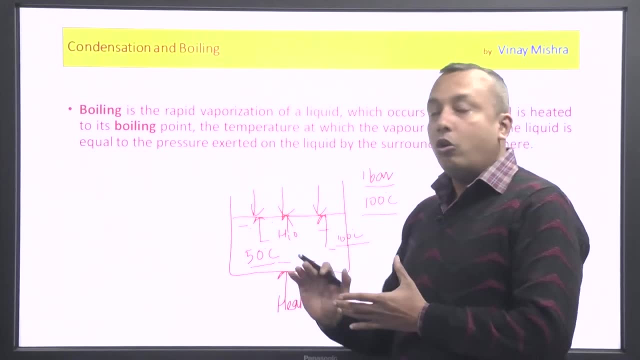 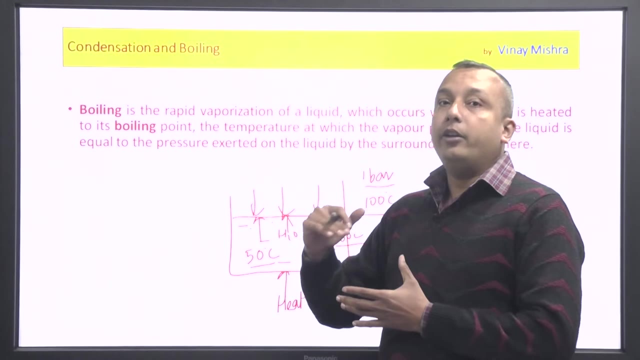 will not get the right temperature. and what will happen? The liquid will not get the correct temperature. now, it will not get the correct temperature. Now we will say that this is basically the vaporization, or this is known as boiling. Now the question is whether it can be boiled at less than 100 degree centigrade or at more than 100 degree centigrade. The answer is yes. It can be boiled at 90 degree centigrade. It can be boiled at 105 degree centigrade. It can be boiled at 105 degree centigrade. What is the temperature condition? It will basically depend on this atmospheric pressure. 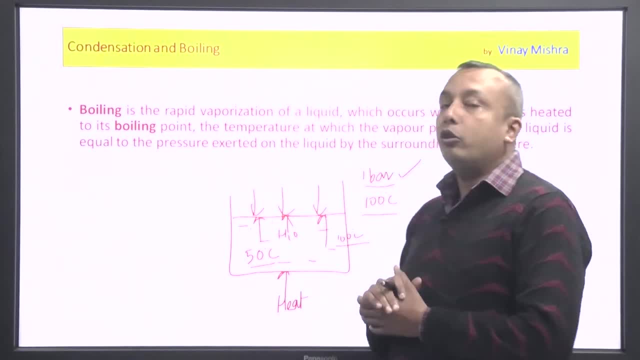 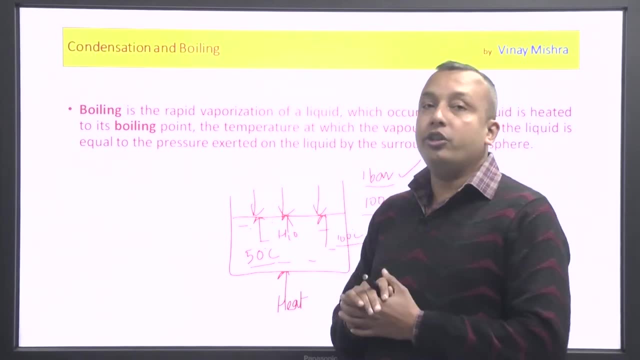 As soon as we increase the atmospheric pressure. for example, we have done 3 bar, So the corresponding saturation temperature of 3 bar will be more than 100.. For example, we have taken 100.05 as the saturation temperature. 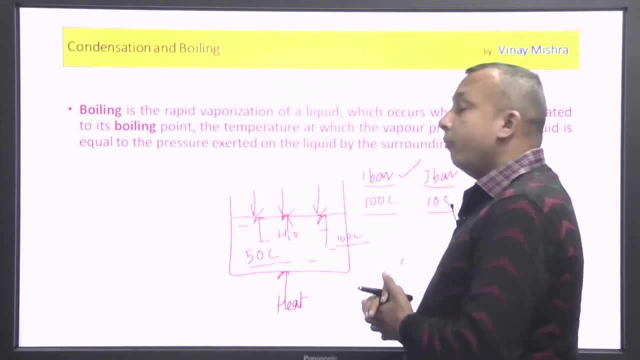 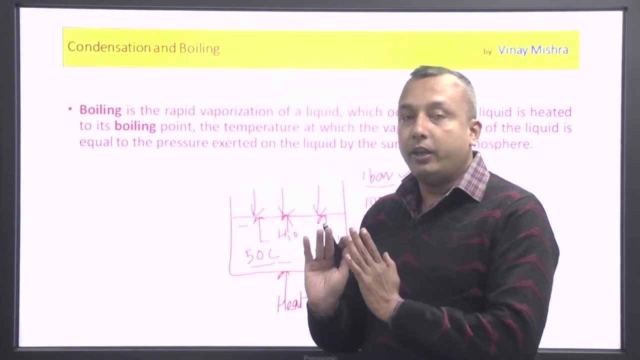 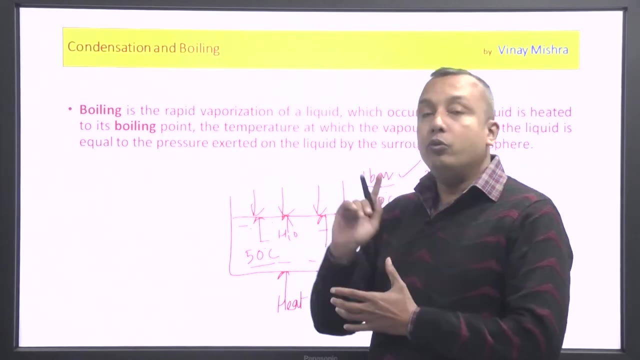 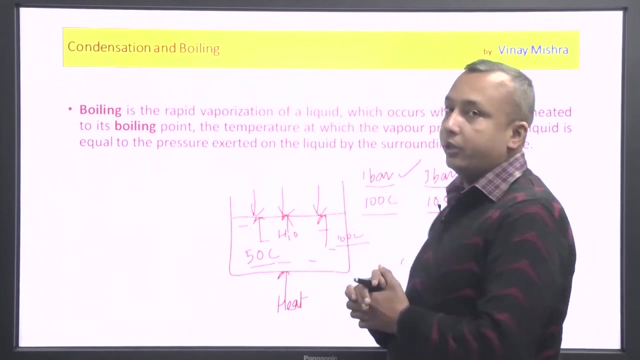 For example. we have to take this example to explain: 105 degree centigrade is done here. If the atmospheric pressure is more than 1 bar, then the temperature of the water here should be equal to the saturation temperature, Which is 105 degree centigrade. 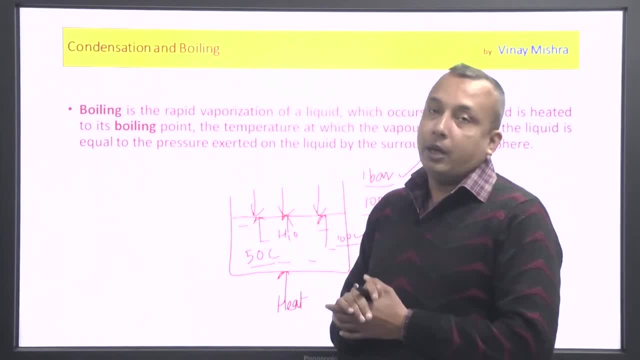 That is, the boiling will start here at 105 degree centigrade. When 105 degree centigrade reaches its temperature, then we will say that the boiling has started here Or the phase transformation has started. 50,, 60,, 70,, 100. 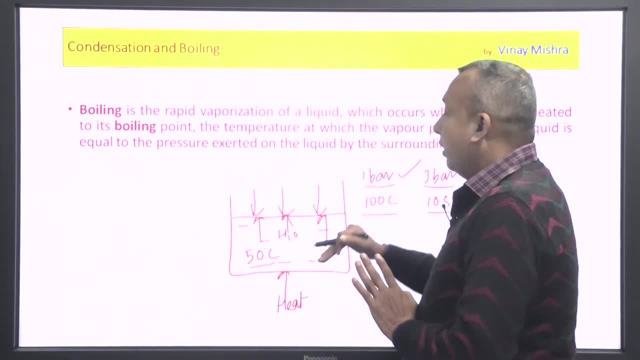 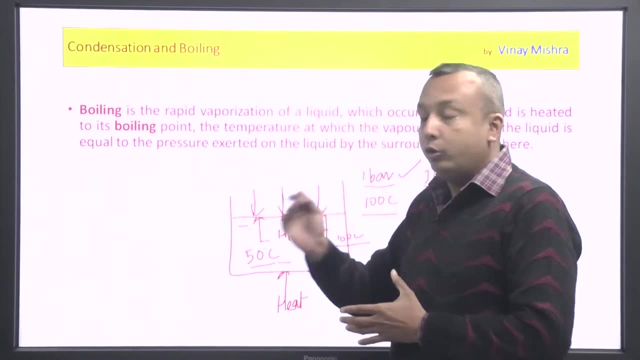 The water will remain at 100.. Why? Because now our atmospheric pressure is basically 3 bar. The corresponding saturation temperature is 105 degree centigrade. So in this way we see that the boiling temperature, the boiling point, can also exceed 100.. 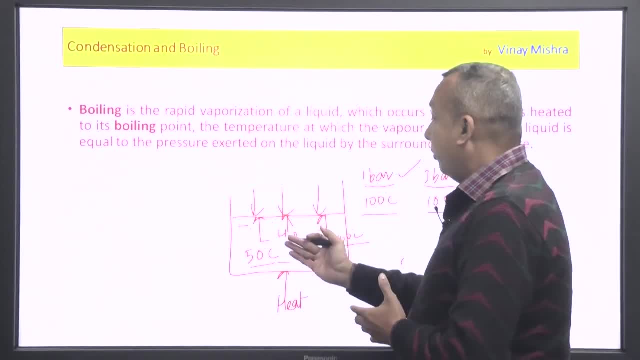 When, When we increase the atmospheric pressure. That is why, when we reduce the atmospheric pressure, for example, we reverse it, then what will happen? Suppose 0.5 bar We have done atmospheric pressure, The corresponding saturation temperature will also be less than 100. 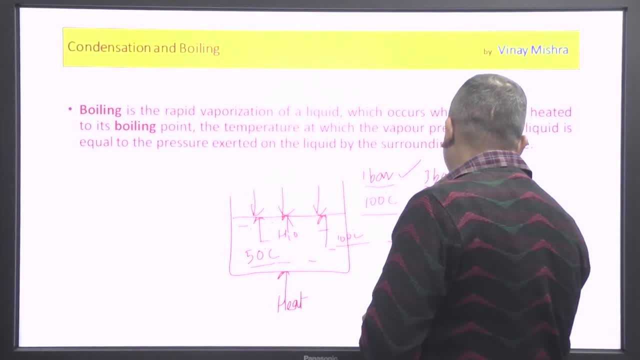 For example, we have said that it is 80 degree centigrade. That is now for 0.5 bar atmospheric pressure. our saturation temperature is 80 degree centigrade. Now the water here, the liquid here, will not boil at 100 degree centigrade. 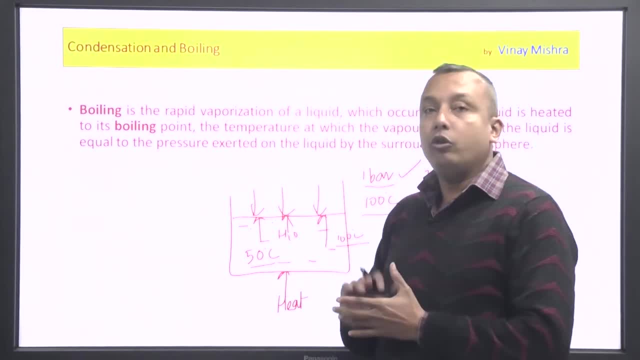 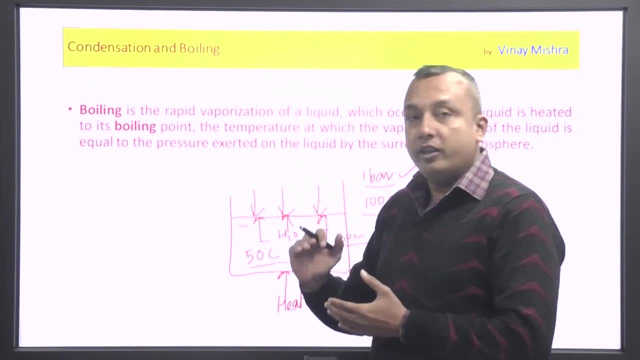 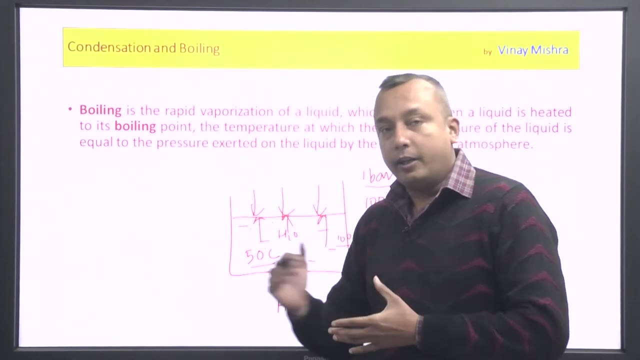 When will it boil? now It will boil at 80 degree centigrade. Why? Because our atmospheric pressure is less than 1 bar 0.5, for example. That is, the molecules will need less energy to escape. That is, the water molecules will keep escaping at 80 degree centigrade. 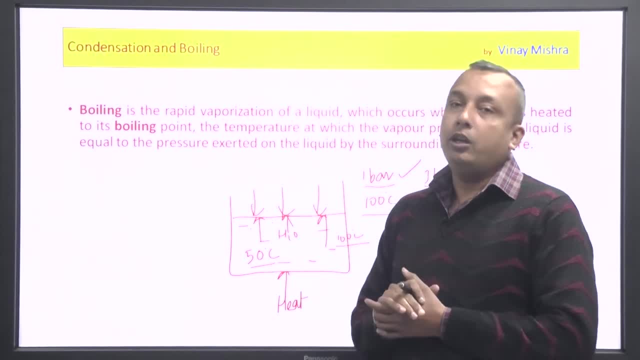 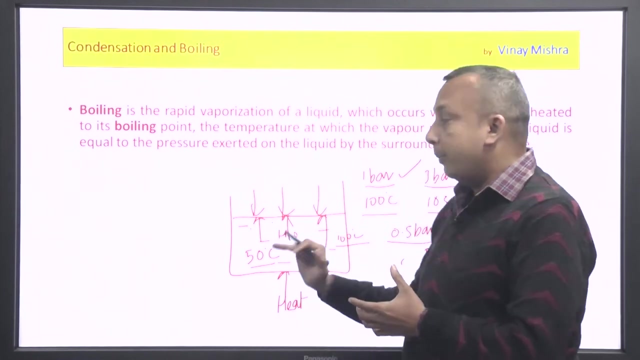 Or our boiling will start, Our vapor transformation will start. So in this way we have seen that the boiling point is basically depending on atmospheric pressure. The corresponding pressure of the atmospheric pressure will be the vapor pressure. So when the vapor pressure will be equal to the atmospheric pressure, then only we will say that our boiling is starting here. 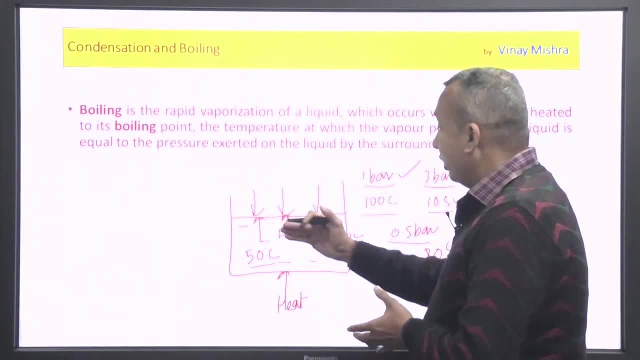 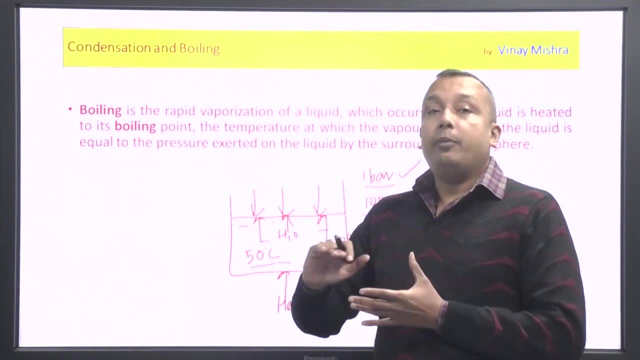 Our evaporation is starting. So in this way we see that when the atmospheric pressure increases, that is, if the water is taken to such a place where the atmospheric pressure is high, then in that condition our water will not boil at 100 degree centigrade. 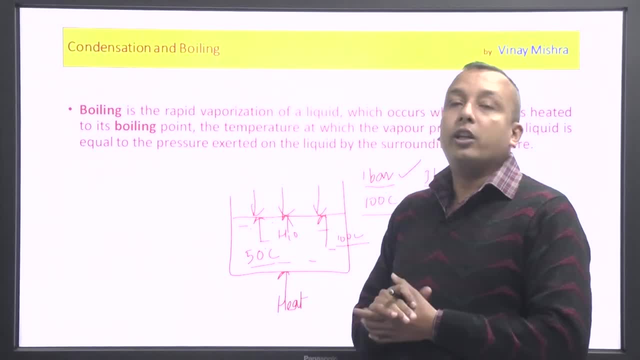 It will be more than 100 degree centigrade. In the case of mountains, we see that our atmospheric pressure is less. there It is a little less than 1 bar. 0.8, 0.9,. we can say in this way: 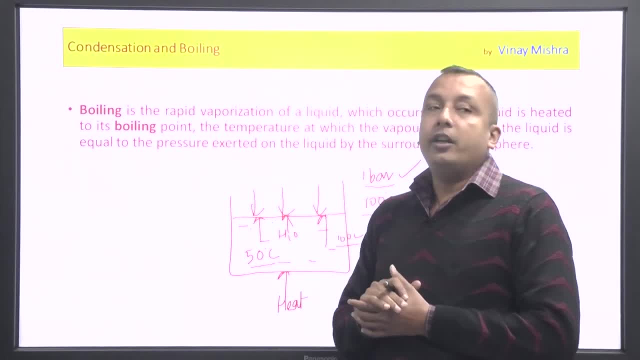 In that condition, the boiling water will not be at 100 degree centigrade, It will be at 90 degree centigrade Or it will be less than 100 degree centigrade, For example. That is why we say that the water on the mountains boils quickly. 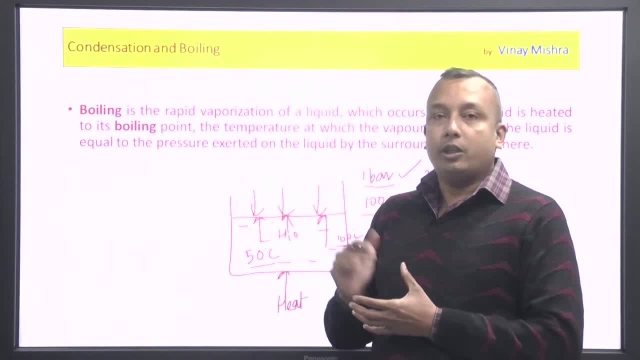 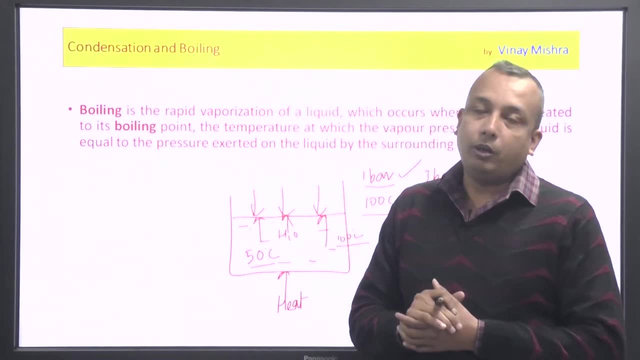 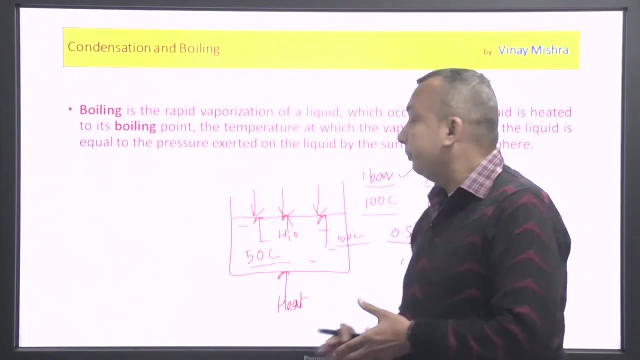 Because the atmospheric pressure is less there. Because of this, our corresponding water will not boil. The value of the vapor pressure is also less. Due to this, the saturation temperature also decreases And the boiling and phase transformation that we have is less than 100 degree centigrade. 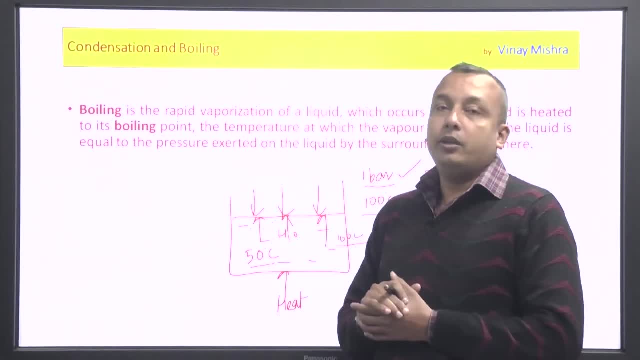 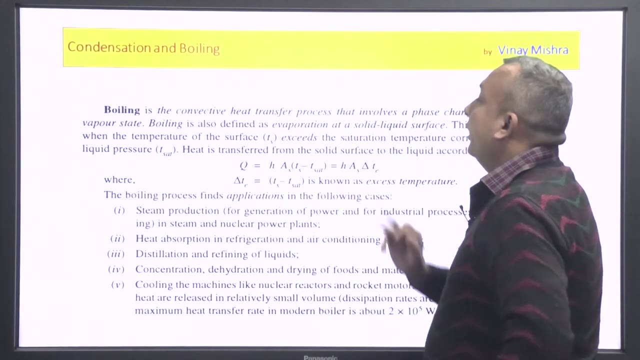 So in this way we have seen that. what is the boiling process and how molecules behave in the boiling process? What is the role of vapor pressure and atmospheric pressure in boiling? Boiling is the convective heat transfer process that involve a phase change from the liquid to vapor state. 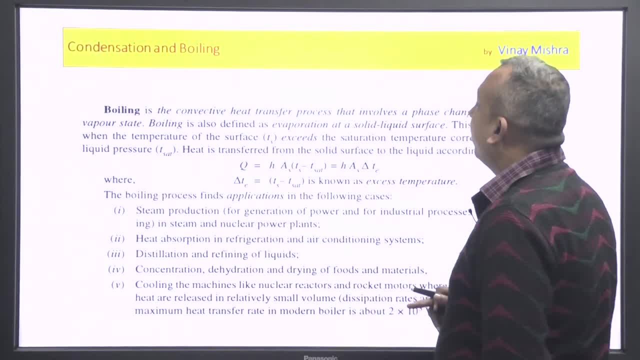 Boiling is also defined as the evaporation of at a solid liquid surface. This is possible only when the temperature of surface Ts exceeds the saturation temperature corresponding to the liquid pressure T saturation. Heat is transferred from the solid surface to the liquid according to the law of this. 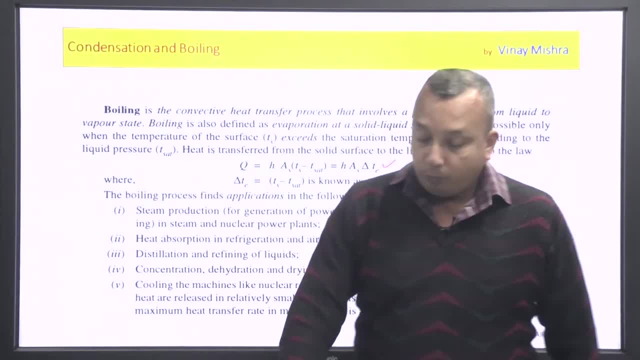 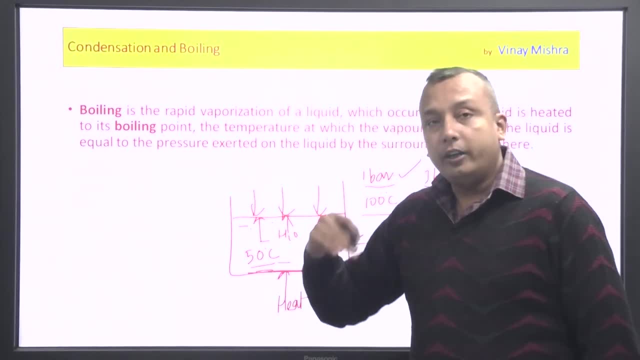 Basically what will happen in the boiling process. If we look at the back Here, the heat is there. Basically, this is our conductive plate. From the conductive plate the heat transformation is happening to the molecules in the liquid. 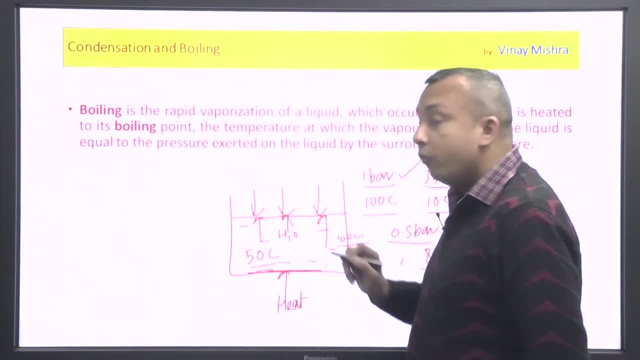 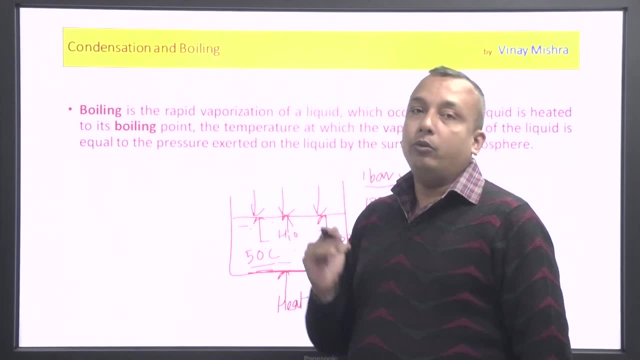 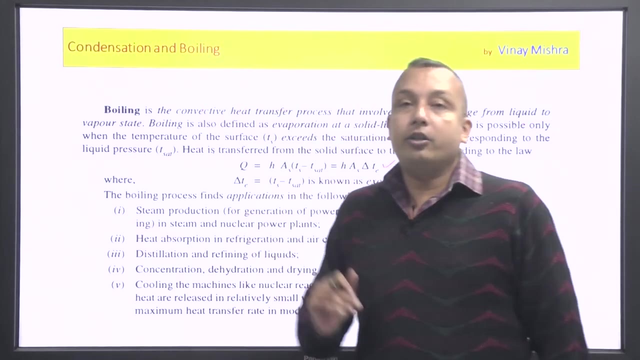 When the heat transformation happens in the conductive plate, in the liquid, In the metal. Now, from there the heat transformation will take place in the liquid phase. That means the heat transformation will take place in this water. So basically, the heat transformation is happening through conduction. 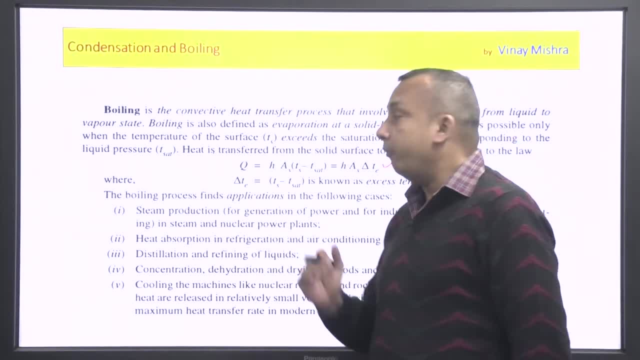 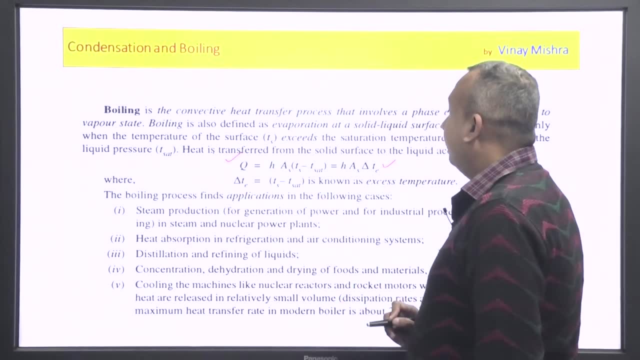 Because first we are giving the heat to the liquid metal And then basically, our convection is happening. So in the case of convection, the heat transfer rate will be H A Ts minus T saturation, which is equal to H A S delta T E. 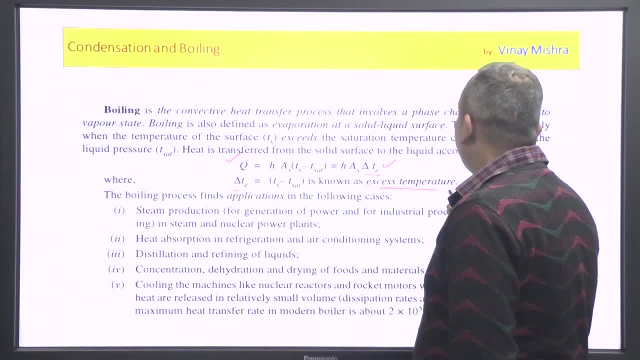 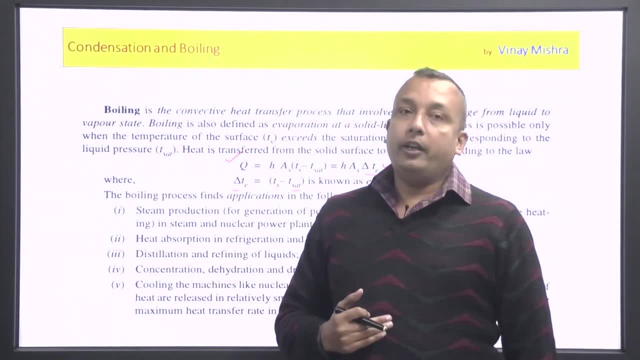 What is delta T E? Delta T E is known as excess temperature, T S minus T. saturation means the temperature of the surface and the temperature of the saturation. In that condition, we will say that the value of T E is the excess temperature. 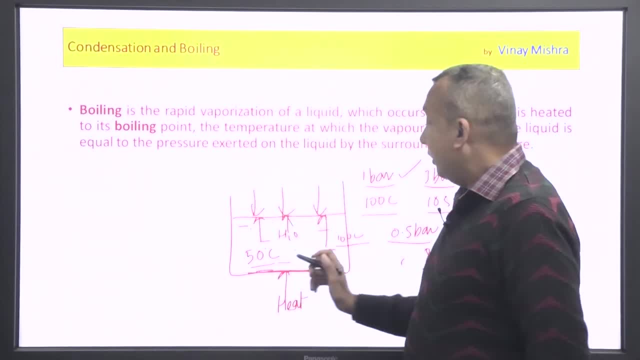 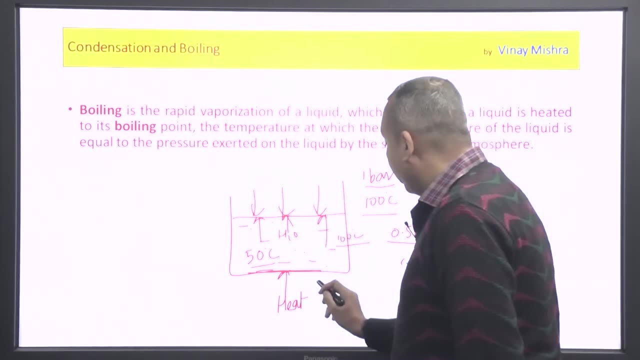 What is the temperature of the excess? What is the meaning of excess? Its saturation temperature is 100. If the temperature of this plate is if the temperature of the surface is 120 degree centigrade and the saturation temperature of the water is 100 degree centigrade. 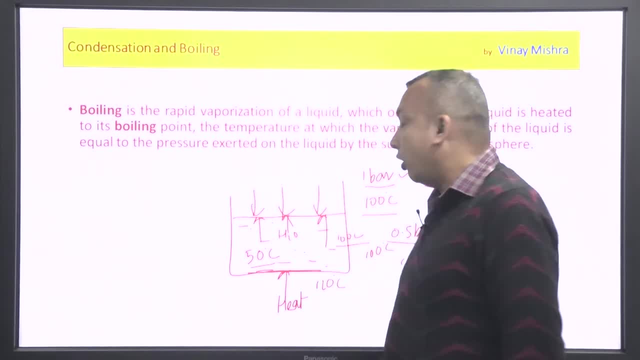 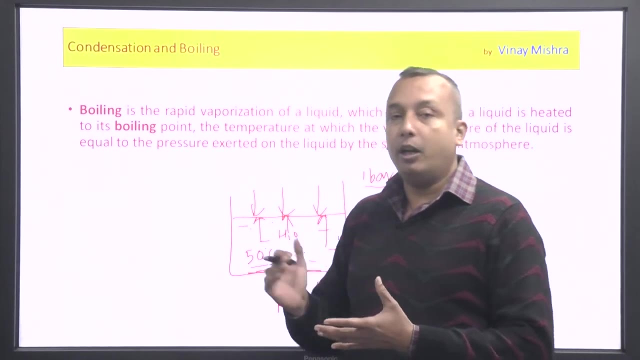 then T excess will be 120 minus 100, which is equal to 20 degree centigrade. That means the temperature of the metallic surface is more than the saturation temperature In the case of boiling. So here we will take the concept of T excess. 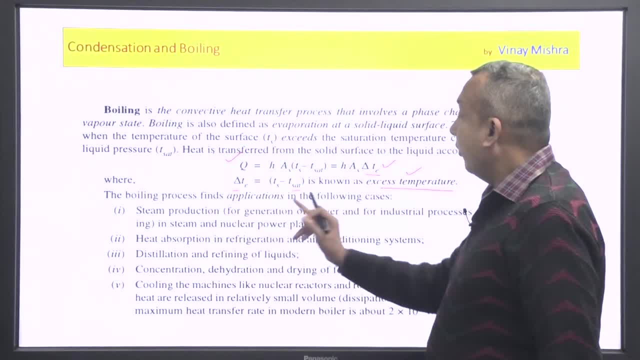 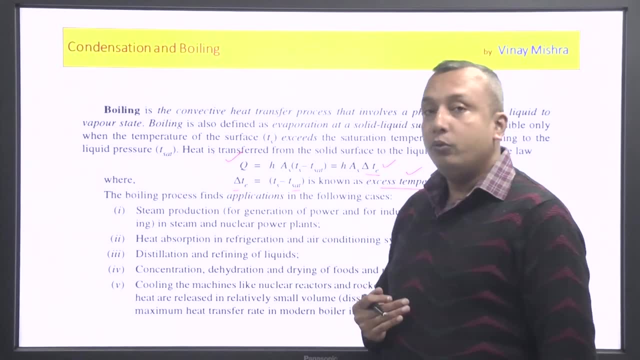 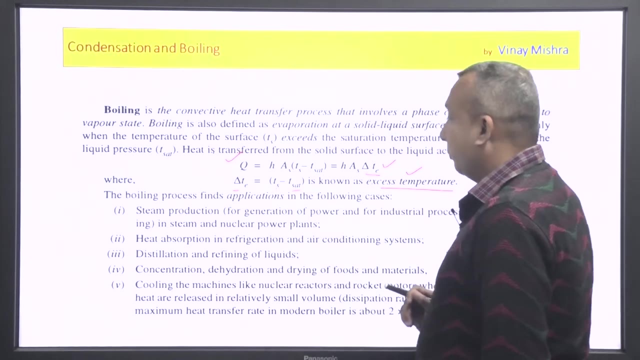 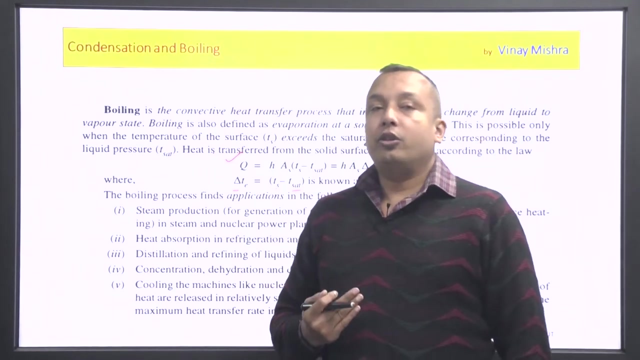 Boiling process finds application in the following cases: Steam production- Where is the use of boiling? Where is its application? Steam production for generation of power for industrial process and space heating in steam and nuclear power plants. That means in steam power plant where the generation of steam is. 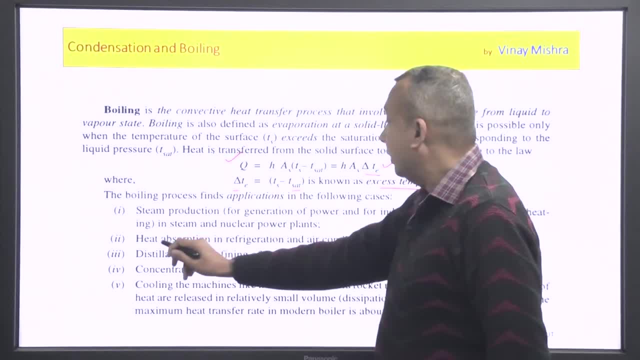 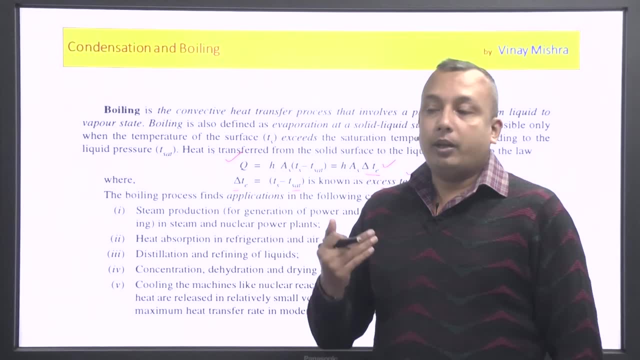 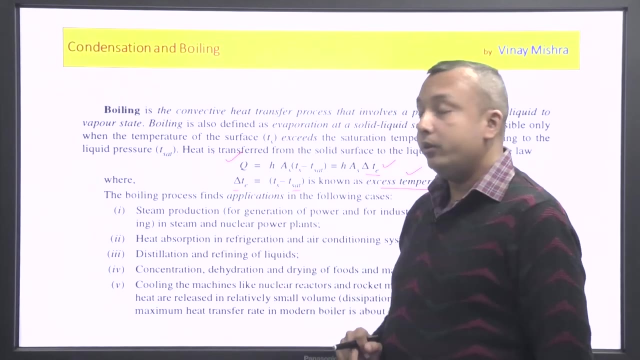 used to make electricity. Heat absorption, Heat absorption in refrigeration and air condition system Absorption in refrigeration industries where we need low temperature- We can use it there. Distillation and refining of liquid Concentration, dehydration and drying of food and material. 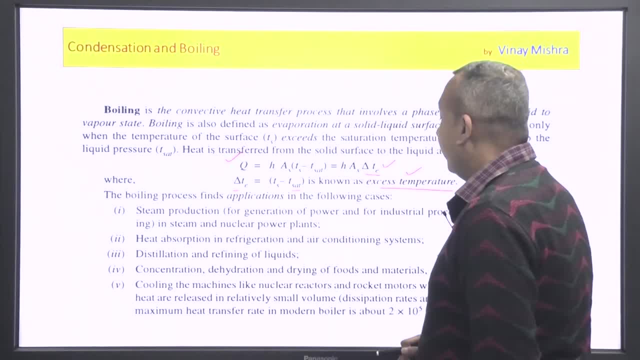 We also use it here, Coaling the machine like nuclear reactor and rocket motors, where the large quantities of heat are released in relatively small volume. Dissipation rate are high as 10 to the power. 8 watt per meter square. The maximum heat transfer rate in modern boiler is about this. 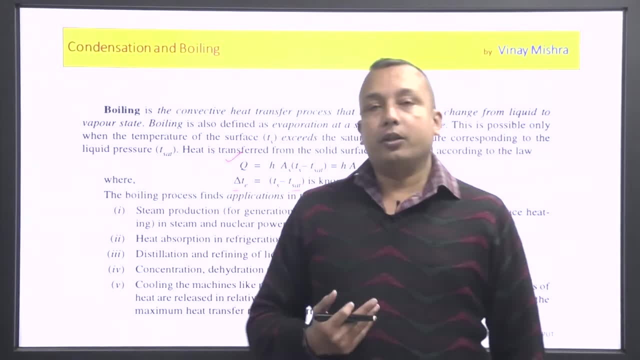 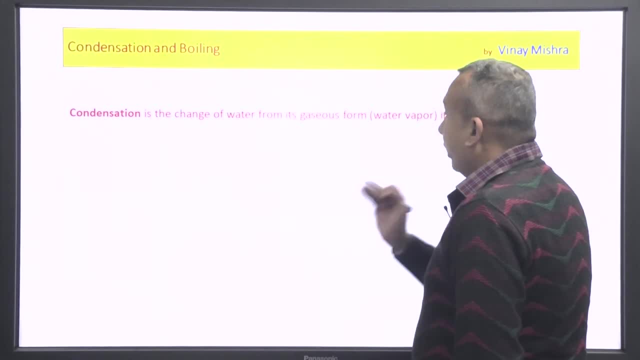 That means basically where we use boiler, we basically use it there. Condensation: What is condensation process? Condensation is the change of water from its gases form- Water vapour- into liquid water. This is the process by which the phase transformation takes place. 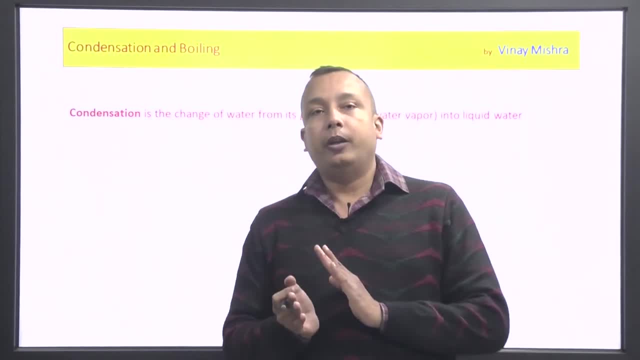 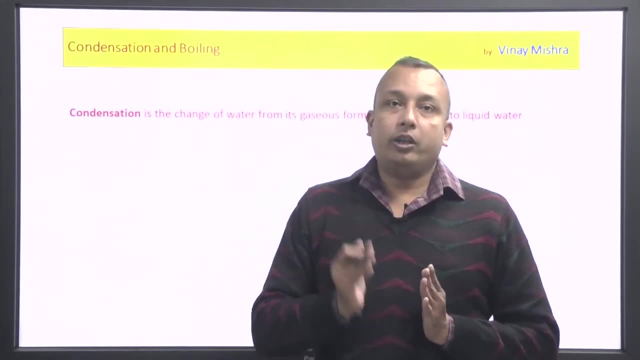 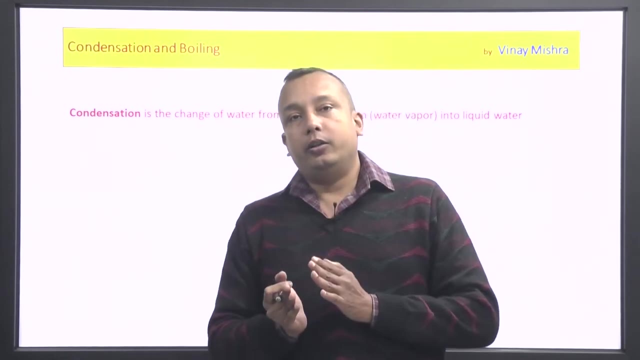 from vapour to liquid form. What happened earlier? What was happening in boiling? From liquid to vapour, From liquid to vapour, phase transformation was happening. What will happen in condensation? basically, Its reverse. That means when liquid will be made from vapour. 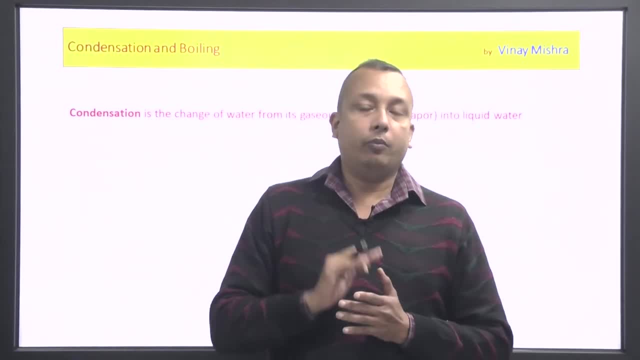 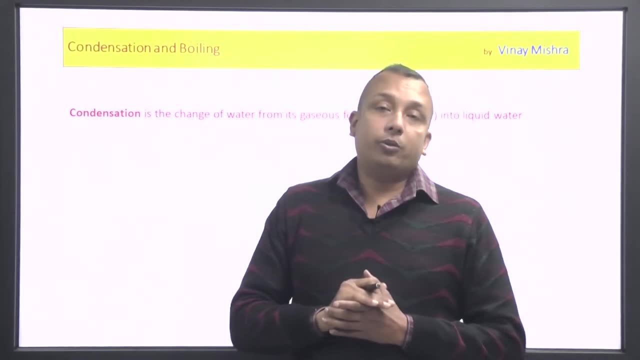 what will we call this process? Condensation process? We will consider it here. We will call it this Now, basically, what happens in condensation, What was happening in vaporization process? We were giving certain amount of heat. We were giving heat. 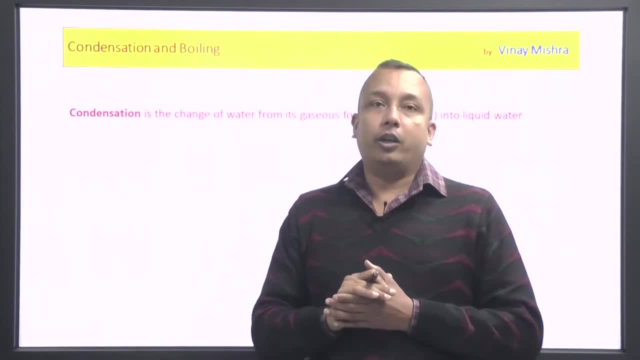 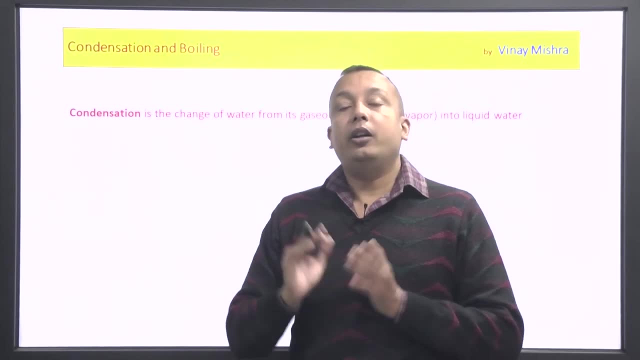 Then the transformation of liquid was happening in vapour. What is the process of condensation? When the transformation of vapour will happen in liquid, then condensation process will happen here. Now, what will happen here? We will have to extract certain amount of heat. 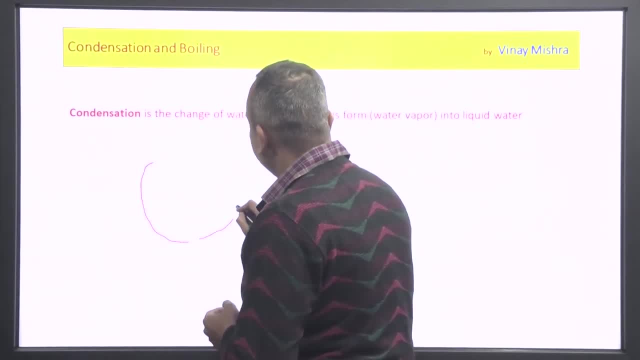 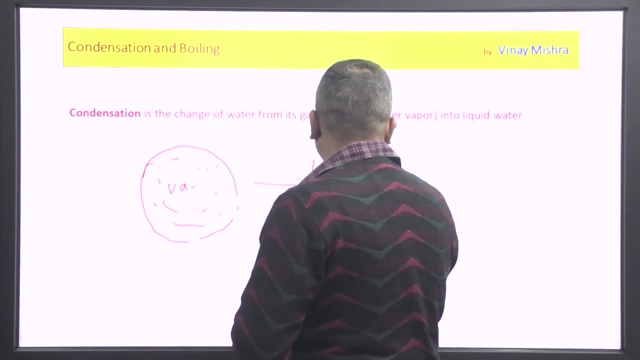 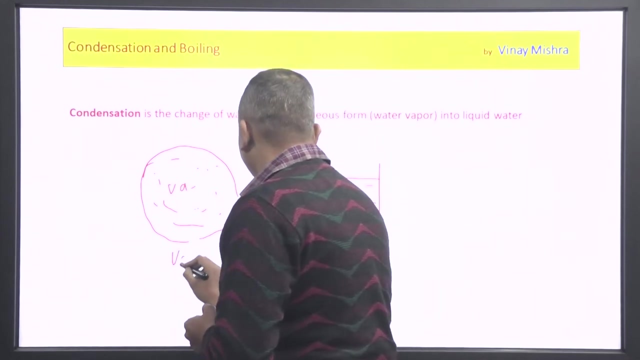 That means this is vapour. This is vapour. We have some droplets. If we take the example of water, then basically this is water, vapour. Its conversion. This is vapour, This is our liquid. That means: 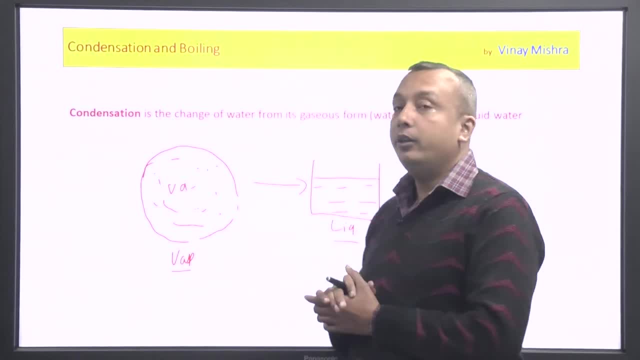 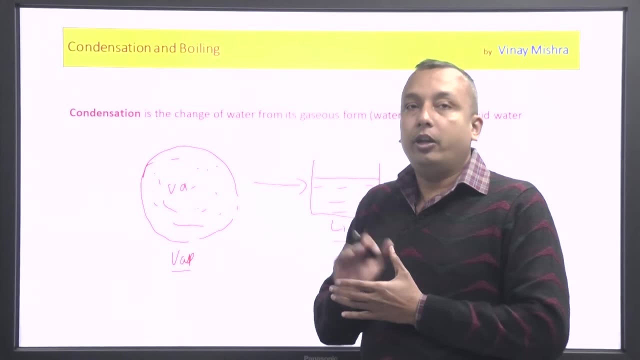 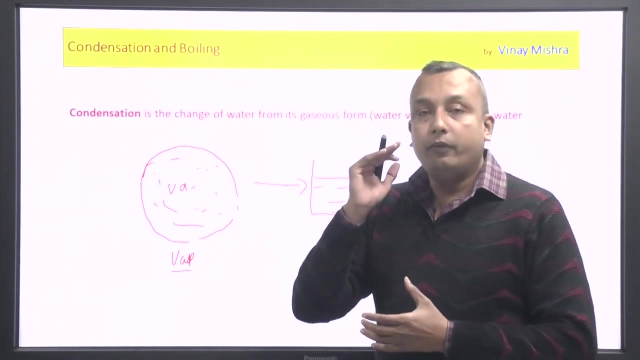 when vapour changes in liquid form. the phase transformation, by which the vapour get transformed into liquid form. this process is known as condensation process. Sorry, This process is known as condensation process. Now, what will happen here? Like in vaporization, 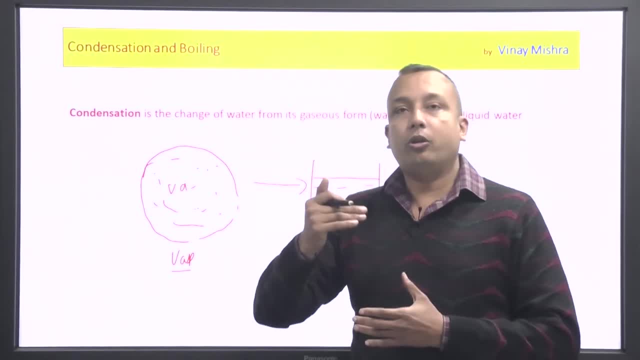 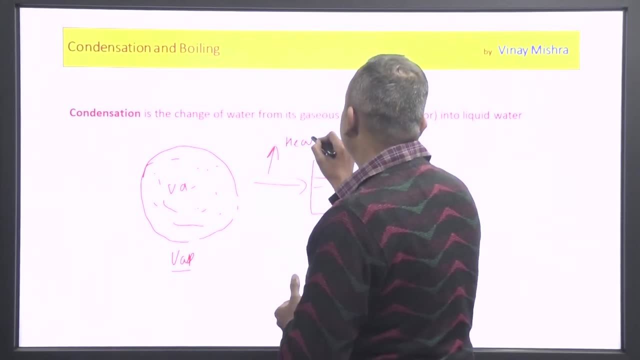 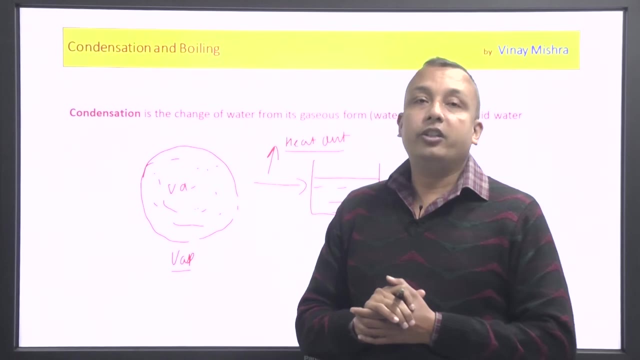 we gave certain amount of heat. What will happen here? We have to extract certain amount of heat. That means we have to extract some heat from here. What will be this amount of heat? What is this? This is the amount of heat which is known as latent heat of condensation. 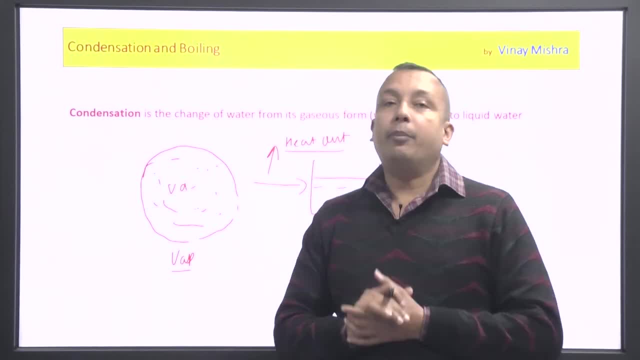 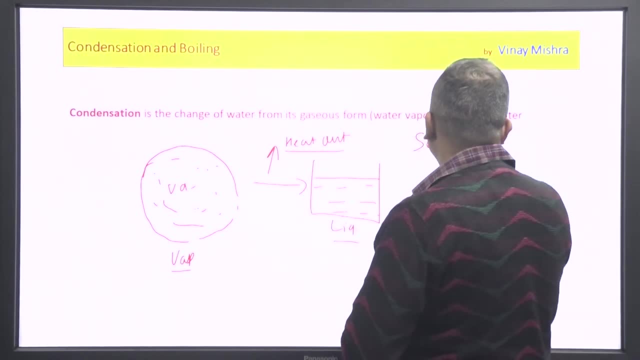 That means? what will we call this? We will call it latent heat, of condensation, Basically. if we see this concept, then basically we have two types of heat. One is your sensible heat and the other is our latent heat. 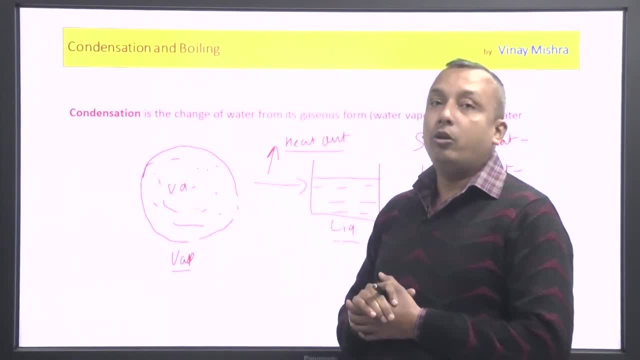 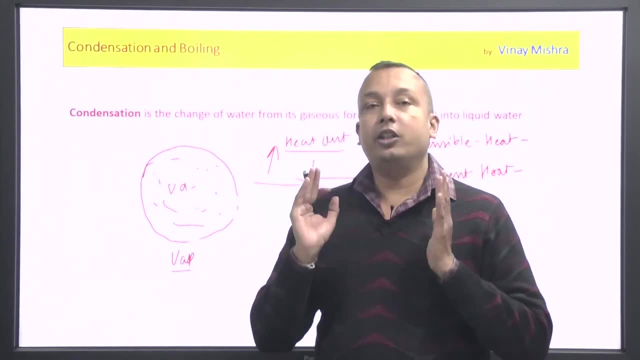 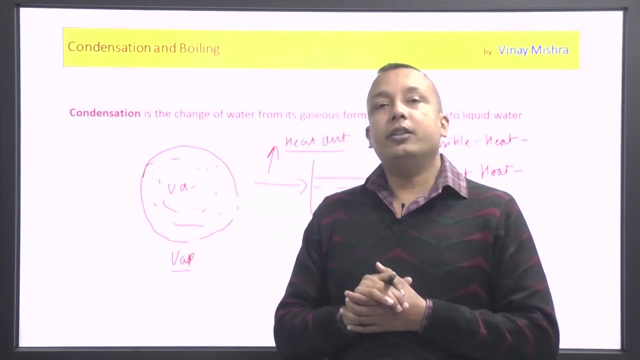 If we talk about sensible heat, sensible heat is the amount of heat which is required to change the temperature in the same phase. That means, in the same phase of any substance, the amount of heat required to change the temperature. we will call this as sensible heat. 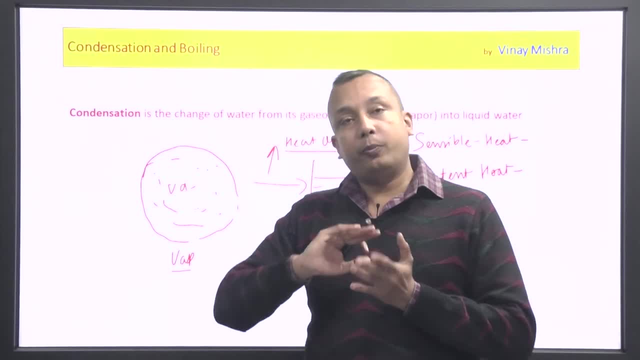 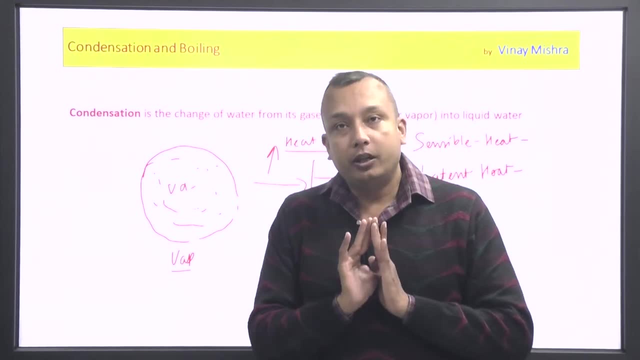 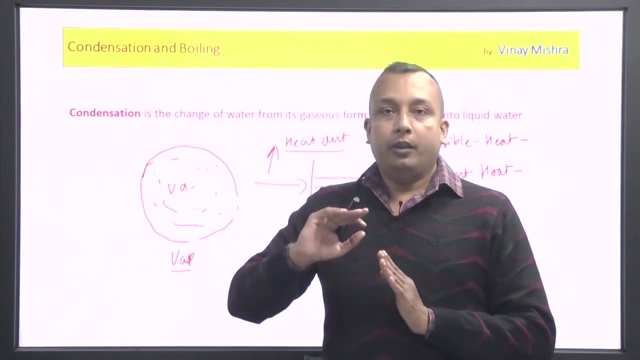 If we talk about latent heat, let us see sensible heat again. Sensibility is the amount of heat required to change the temperature in the same phase. That means the phase is not changing, is liquid and vapour is vapour. reverse it in latent heat. latent heat is the amount. 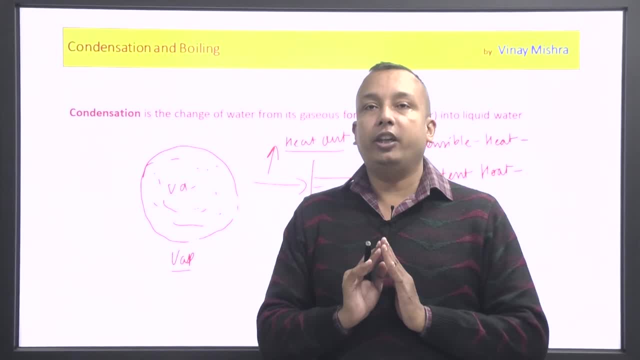 of heat required to change the phase at constant temperature means when the phase is transformed from liquid to vapour or vapour to liquid at constant temperature, then concept of latent heat comes there. So here, basically, latent heat is the amount of heat required to change the phase at the 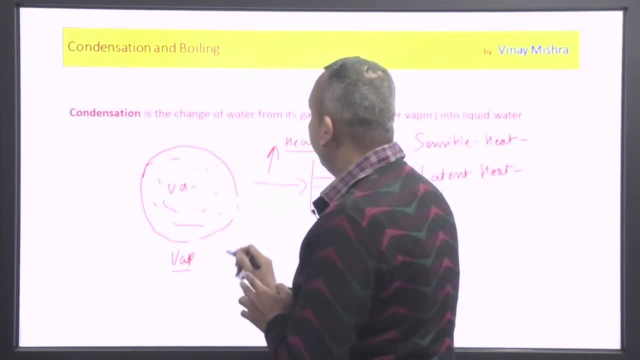 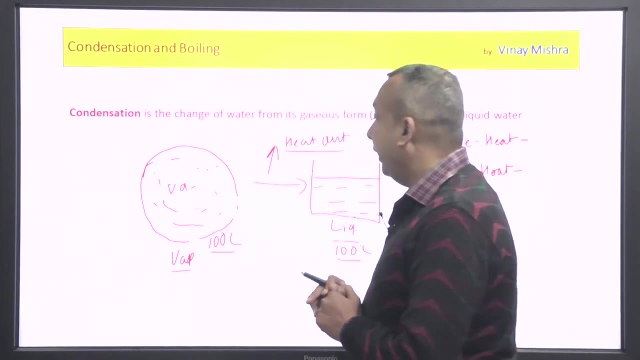 constant temperature means if the temperature here is 100 degree centigrade, its temperature is also 100 degree centigrade. this is vapour. this is liquid. to make liquid from vapour at 100 degree centigrade, the amount of heat extraction will be the amount of heat we. 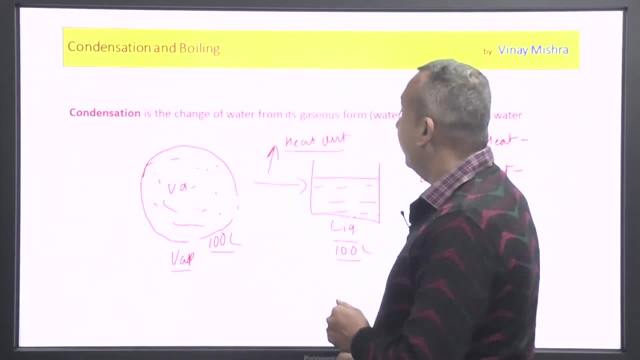 will extract the amount of heat we will remove from vapour. that will be our latent heat. latent heat: Here we have to change the phase at constant temperature. Here, see here the important thing is that the conversion of vapour is happening at. 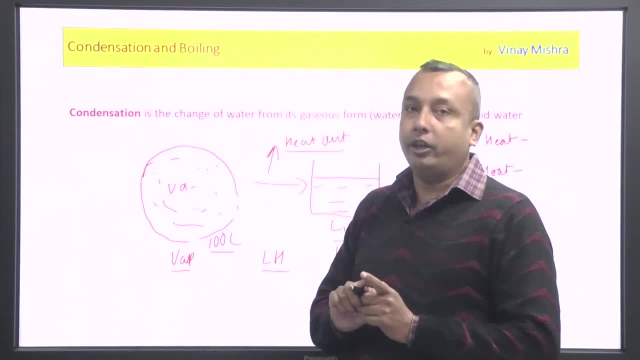 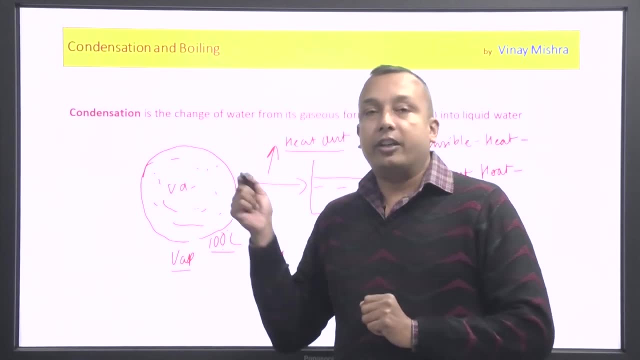 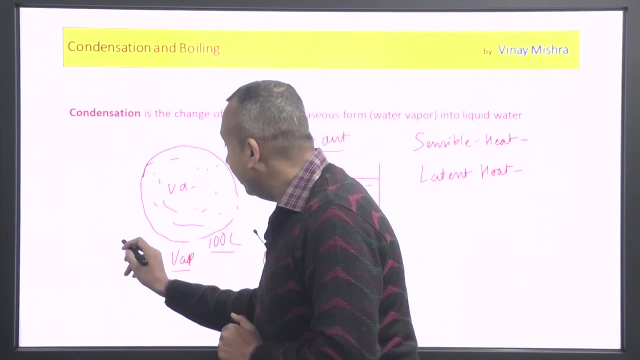 100 degree centigrade in liquid means the temperature is constant. the temperature is constant means basically here, at constant temperature, the heat extraction is happening and that heat is being called latent heat. For example, its temperature- suppose it is 60 degree centigrade- saturation temperature. 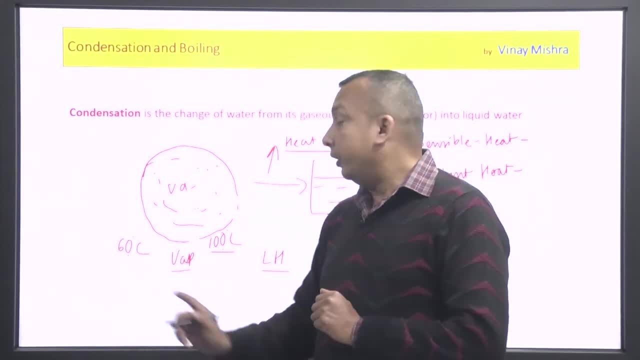 is 100 degree centigrade, Initial temperature. suppose 60 degree centigrade. Suppose we assume that it is 60 degree centigrade or 160 degree centigrade, then firstly what happens is if the temperature of vapour is 160 degree centigrade and saturation temperature: 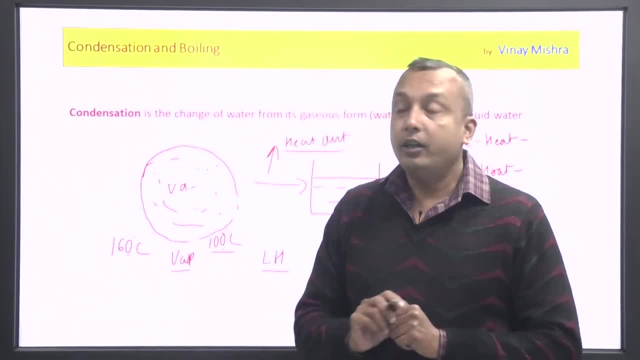 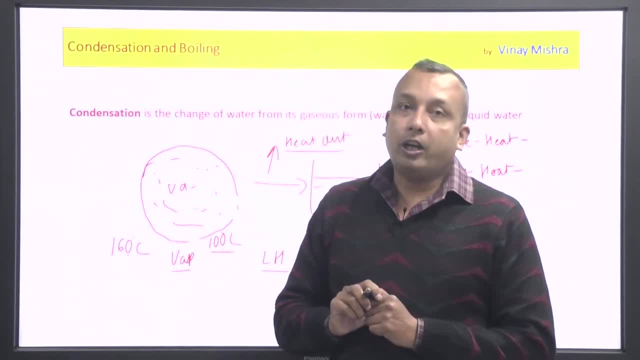 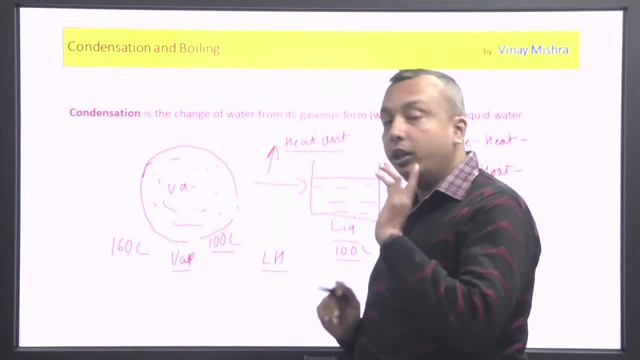 What will be the meaning of sensible heat here? What will be the meaning of sensible heat here? What will be the meaning of sensible heat here till 100 degree centigrade? Vapor is at 160 degree centigrade. It will have to cool down till 100 degree centigrade. 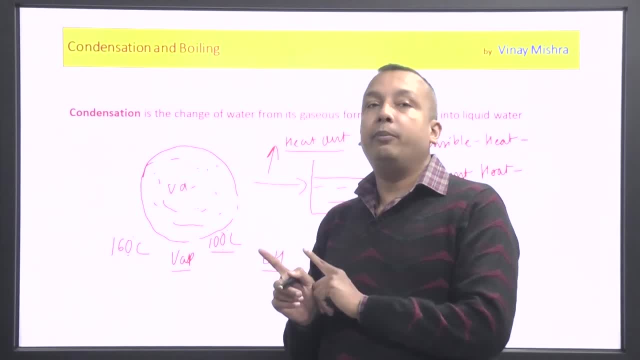 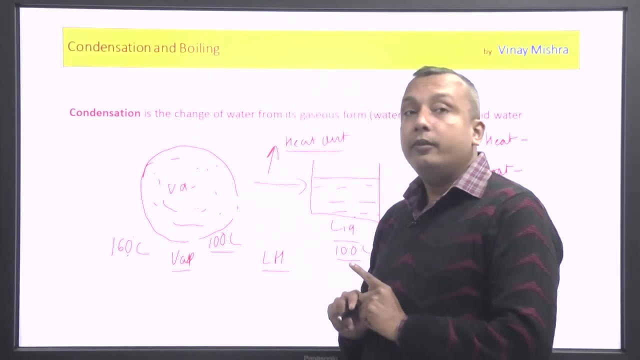 That means the phase of vapor between 160 to 100 degree centigrade is vapor only. That means the phase of vapor between 160 to 100 degree centigrade is vapor only If temperature is changing in same phase, then the interaction of heat will be called as sensible heat. 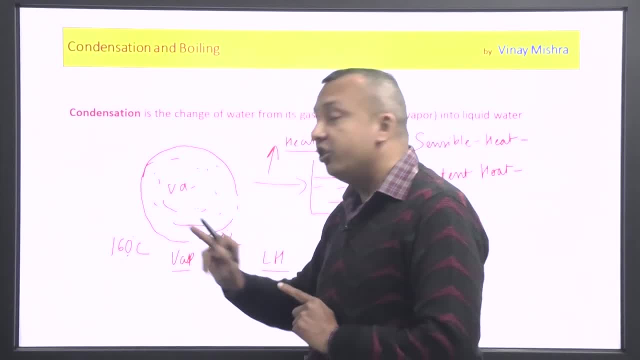 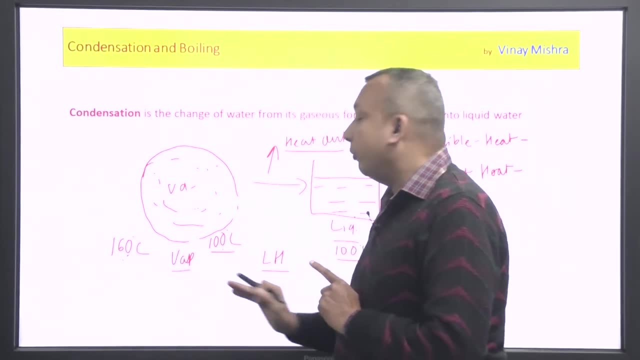 That means in vapor phase itself. we have to change the temperature of 160 degree centigrade to 100 degree centigrade in same phase. In that case, we will say that this is the amount of heat required, which is known as sensible heat. 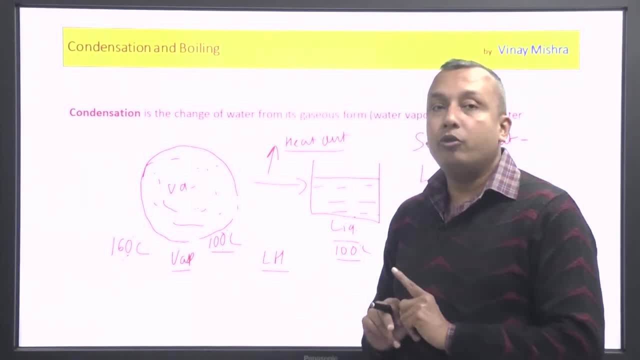 Now it has reached vapor at 100 degree centigrade. When it has reached vapor at 100 degree centigrade, then when it will change in liquid at 100 degree centigrade, then it will change in liquid at 100 degree centigrade. 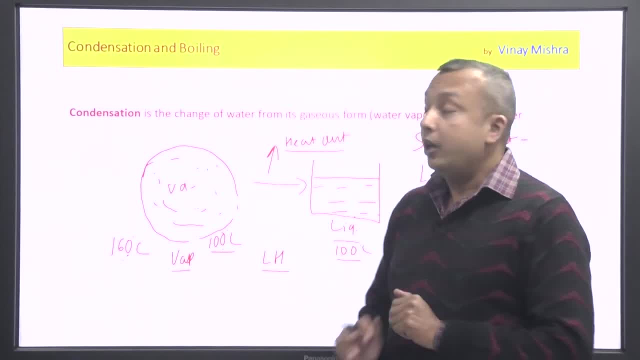 So we will call the heat which we will remove as latent heat. Now, what we have left here? We have left liquid at 100 degree centigrade. We call it as water If we have left liquid at 100 degree centigrade. 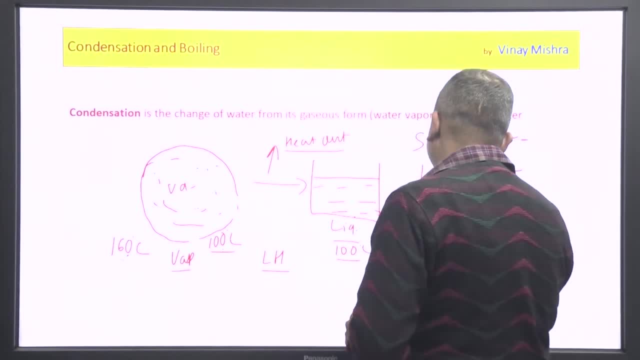 then we have to cool it down more. We have brought it till 50 degree centigrade. Now what has happened? Our water has reached 50 degree centigrade. We had talked about sensible heat at 160 to 100 degree centigrade. 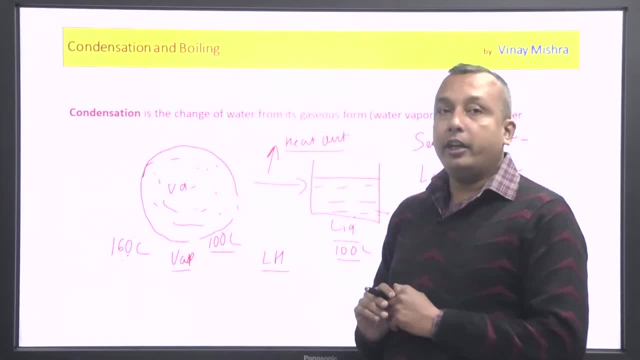 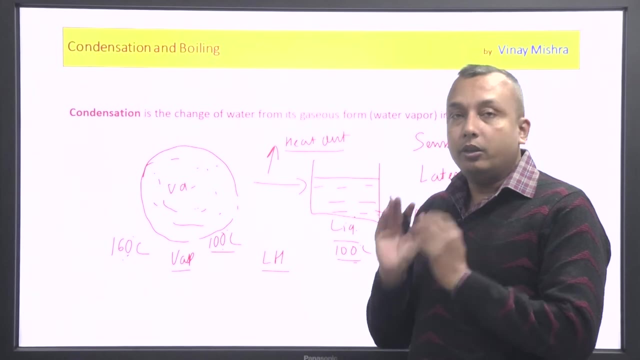 Here we have cooled it down more, from 100 to 50 degree centigrade. Now we will see that the liquid is liquid, but its temperature has changed. So the heat contraction which is happening in the change of temperature, we will call it as sensible heat. 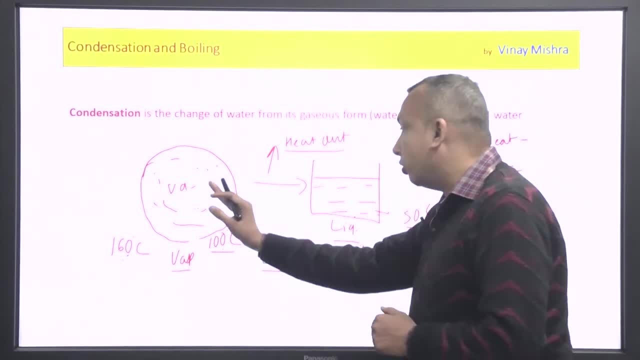 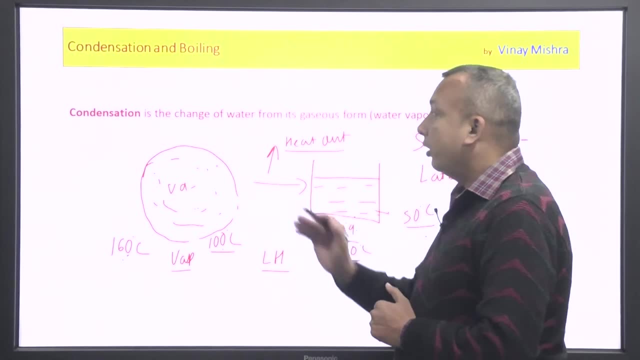 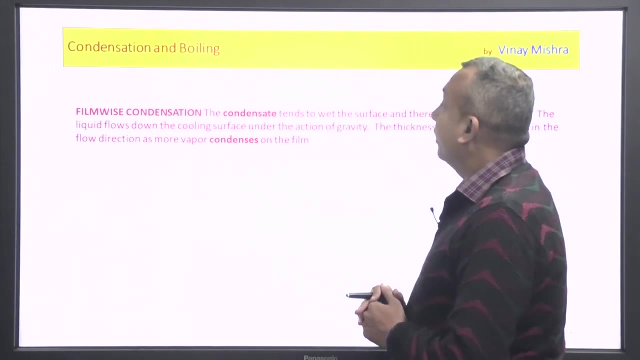 So what will be the concept here? We will call it as sensible heat And this process, which is called as constant temperature, phase transformation, we will call it as the condensation process: Film condensation. Film condensation- Condensate- tend to wet the surface and thereby form a liquid film. 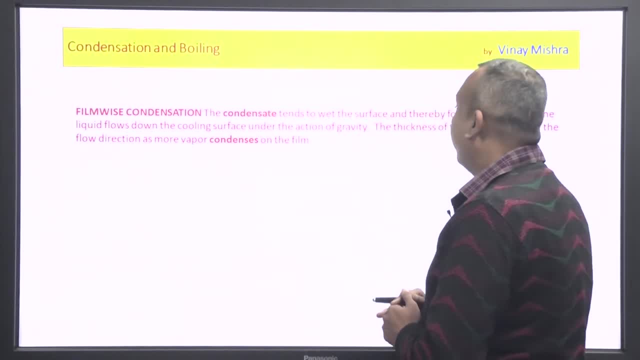 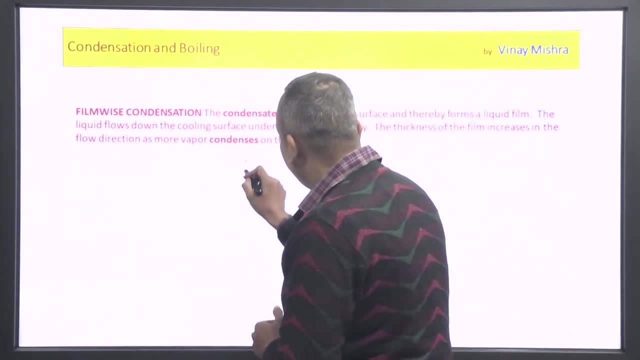 The liquid flows down the cooling surface under the action of gravity, The thickness of film increase in the flow direction as more vapour condensate on film. If we take an example like we have, is this a surface? Is this a surface? 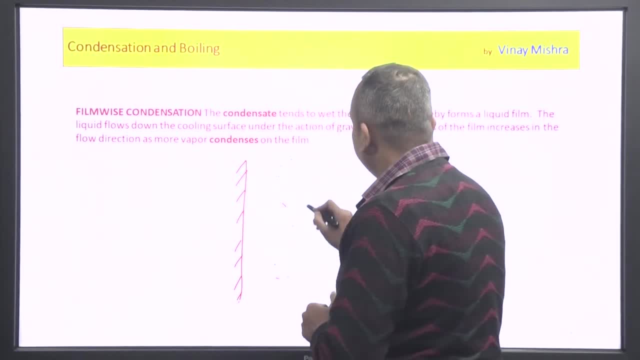 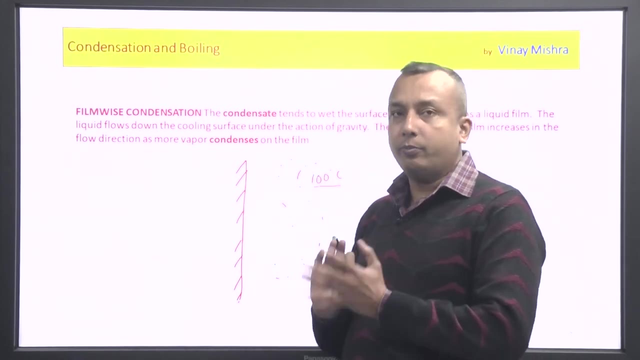 Here there is vapour. For its convenience, we are considering it as 100 degree centigrade saturated vapour. Assume that it is a vapour, water vapour, Its saturation temperature is at 100 degree centigrade or around it. 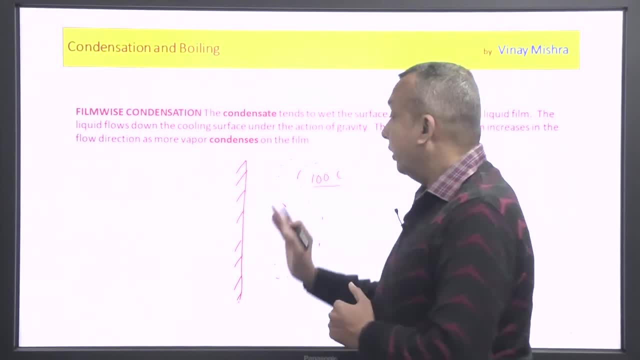 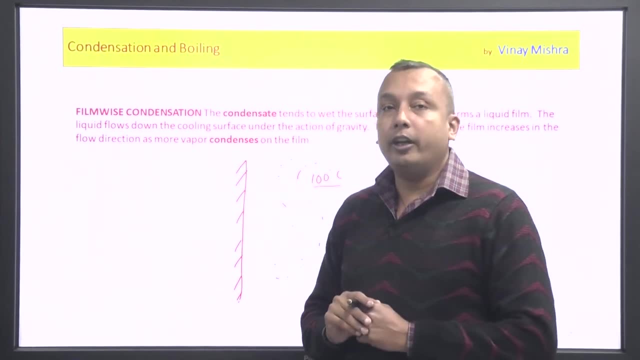 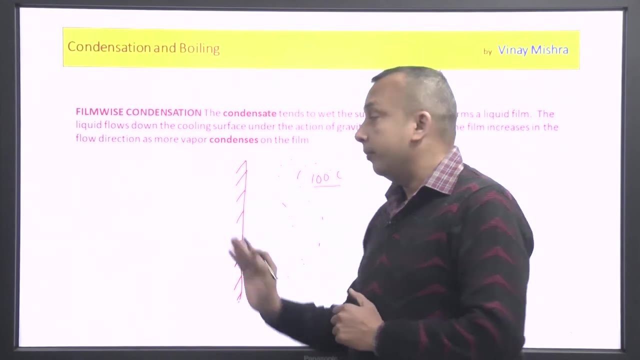 We are talking about vapour. Now what will happen here As soon as it will contact on this surface? As soon as this vapour will contact on this surface and its temperature is low from saturation temperature, its temperature is at saturation temperature. 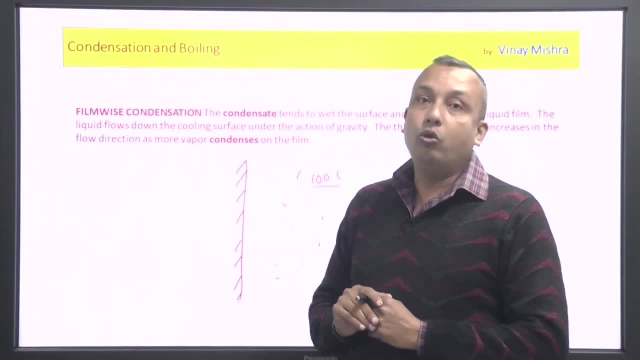 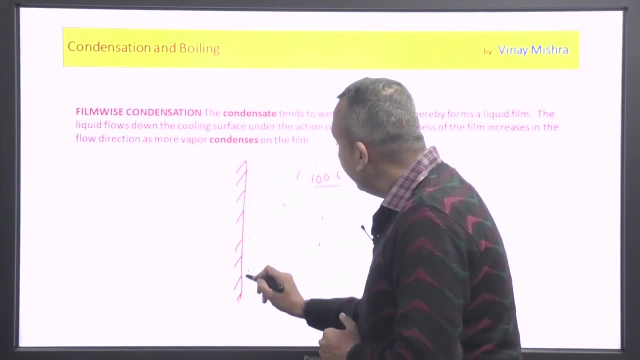 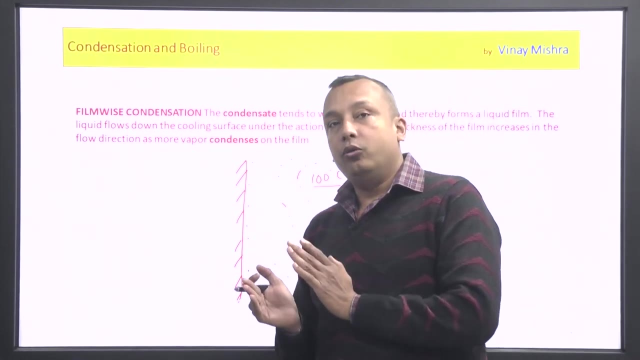 its temperature is at less than saturation temperature. So what will happen, This vapour, saturated vapour, when it will come in contact? when it will come in contact with this surface, then condensation will start. That means vapour will change in liquid form. 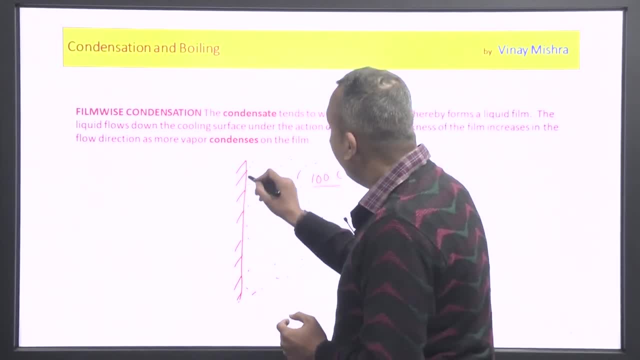 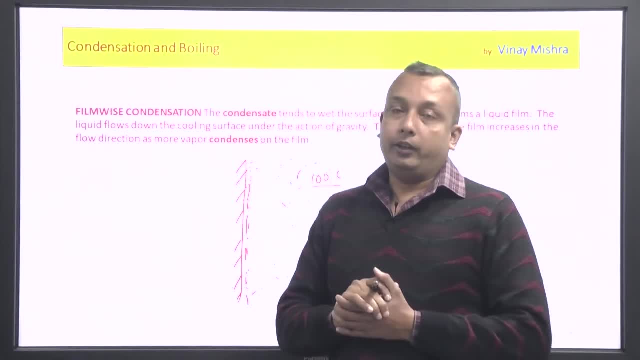 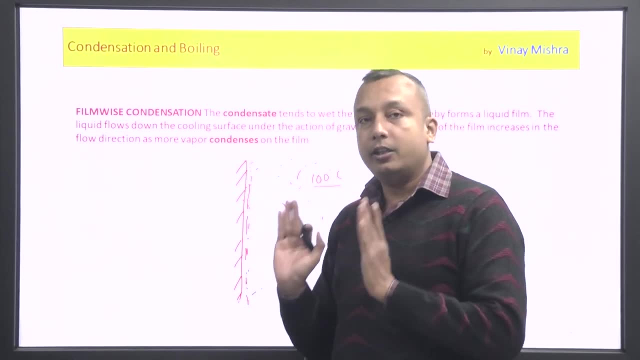 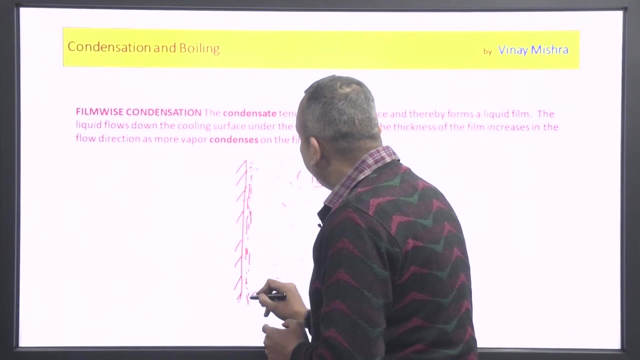 In this way, here a film will form. That means this water will wet this surface completely. It will wet this surface completely. Now what will happen? Basically, a film will form here And molecules are coming. Now film is forming. 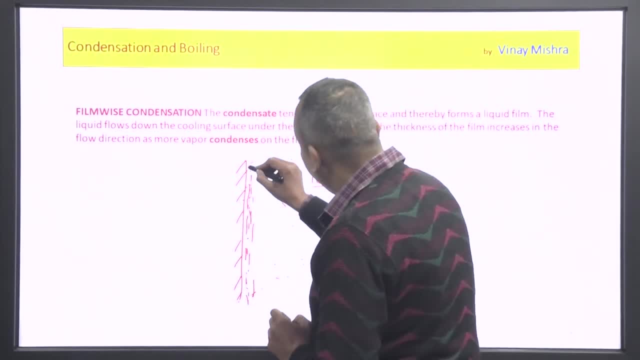 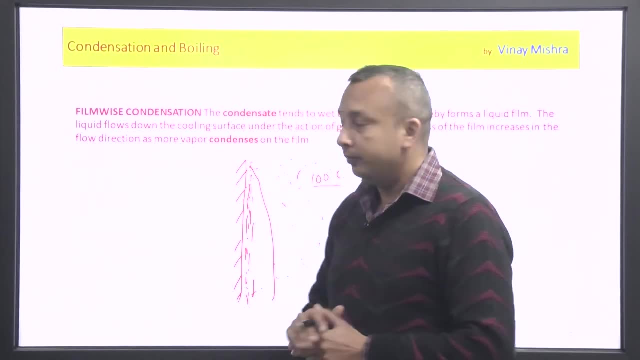 Now its thickness will increase. A layer will form in this way: Now, if we draw the profile of the layer, then it will come in this way: Thickness will keep increasing due to gravity. That means here the thickness of the film. 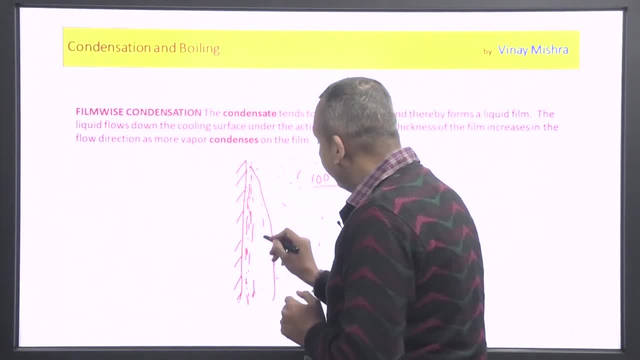 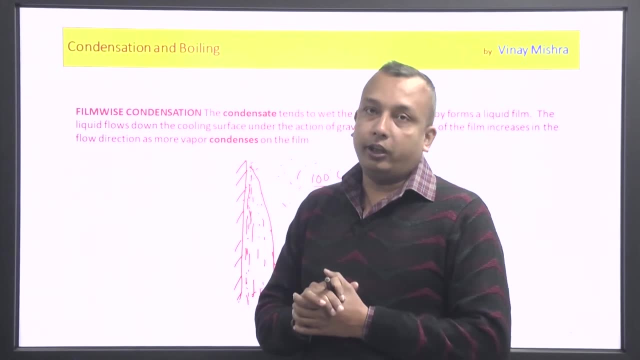 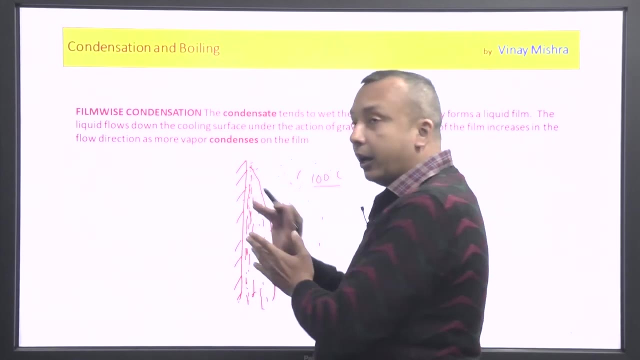 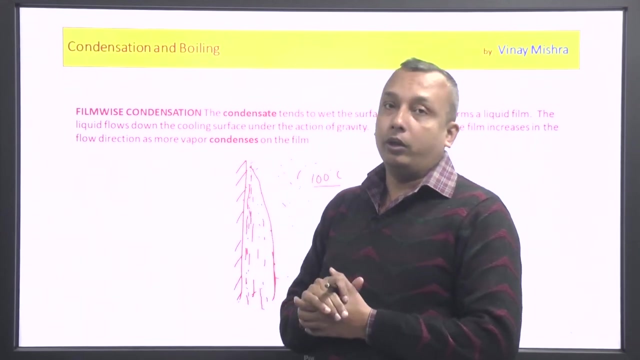 if we draw the curve, then it will keep increasing here And here the curve will come. in this way, Thickness will keep increasing due to gravity. Now, what will happen Now if there will be up-condensation? now, what will happen if vapour will come in its contact? 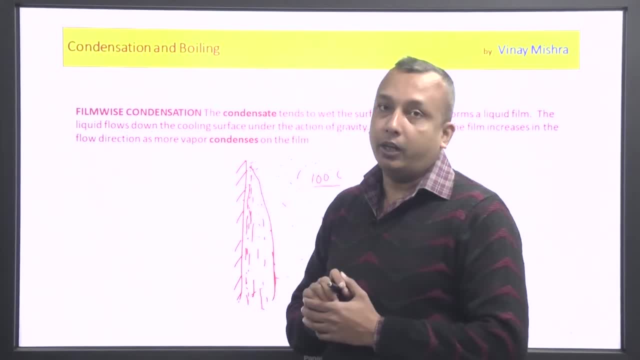 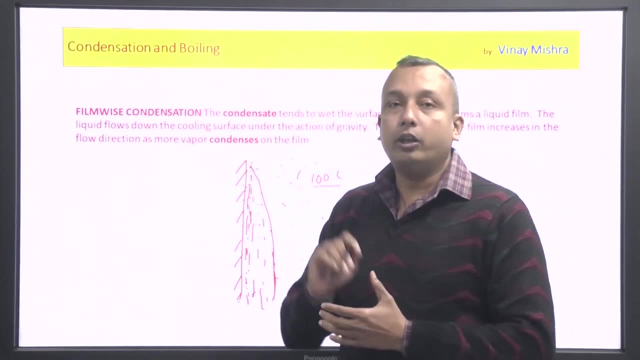 Now see, it had to come in the contact of its surface, But now film has come in the middle. Due to the coming of film, the rate of condensation here becomes less, Or the transformation of heat becomes less. 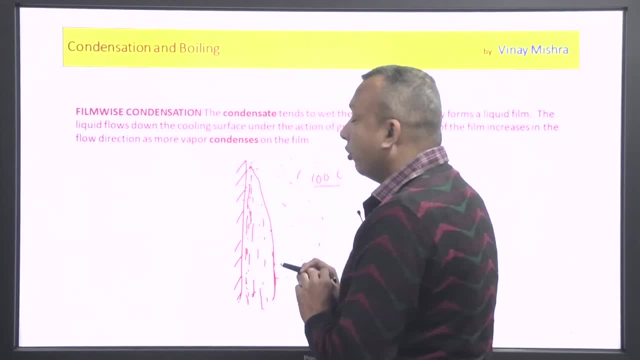 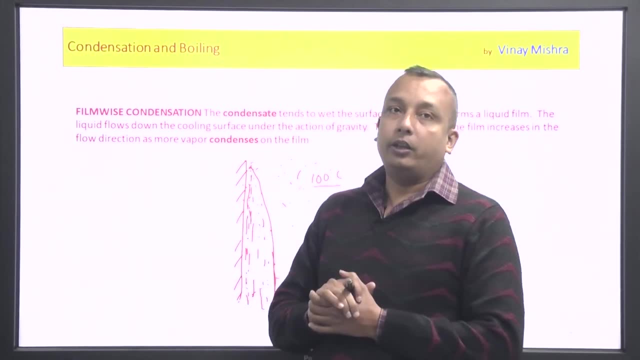 Vapour will come. There will be no contact of this surface. Who will it contact with? It will contact with this film. So whatever condensation happens in this way, then here, basically, we say this is film-wise condensation process. 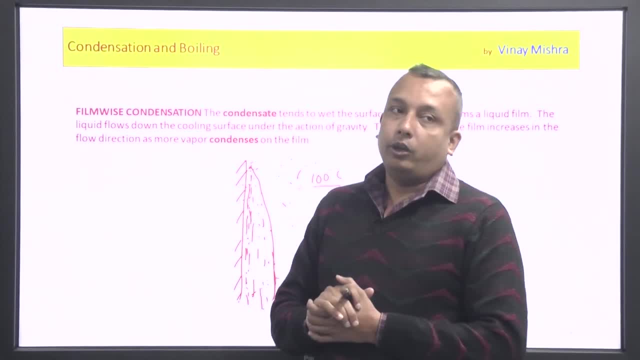 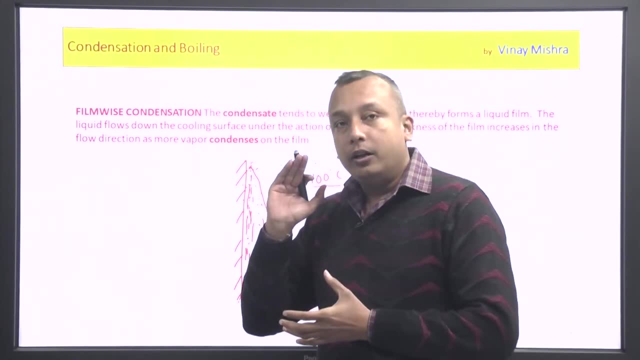 And here the profile will be made. basically, it will be something like this. So here, basically, the condensation will be something like this. It will be film-wise In this. it will wet the surface. That means the droplets will not be made here. 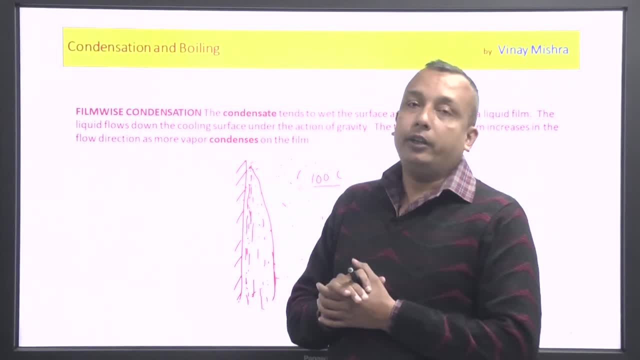 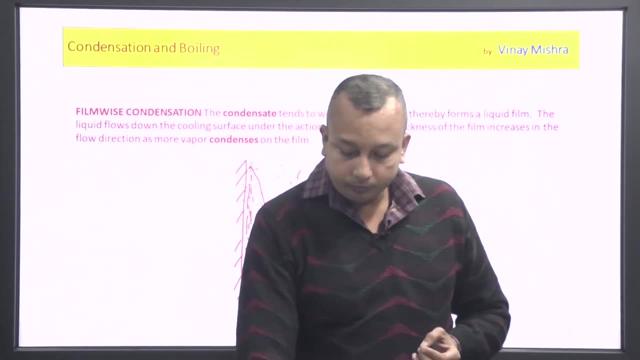 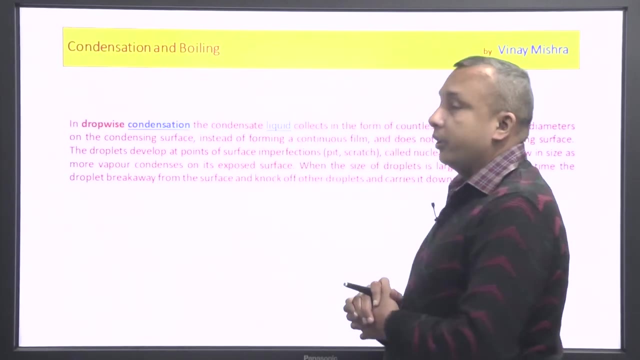 It will wet the surface And here a film will form. So in this way, whatever condensation process will happen, we will say this is film-wise condensation. If we talk about drop-wise condensation, drop-wise condensation process happens in some different way. 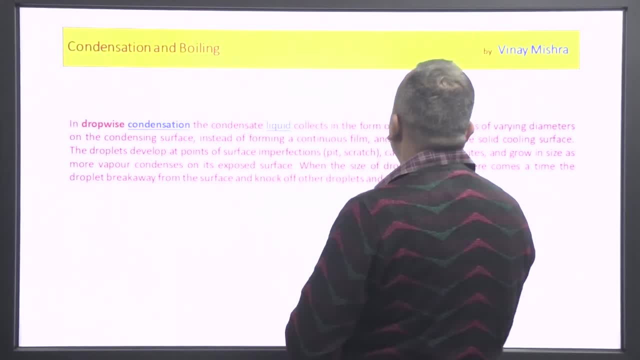 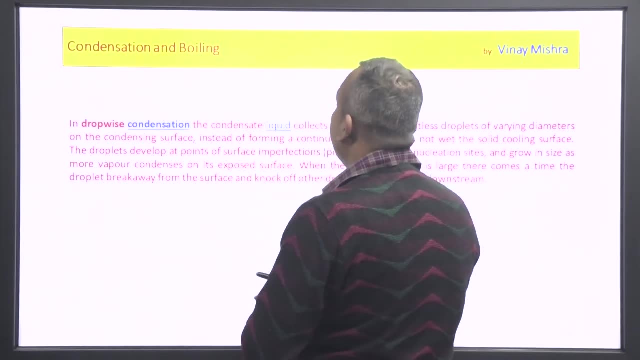 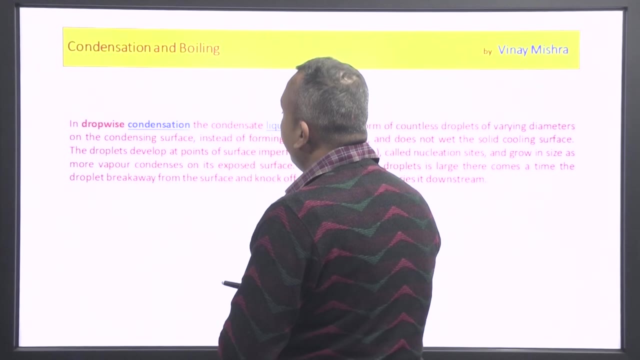 In drop-wise condensation, the condensate liquid collect in the form of countless droplets of varying diameter on the condensing surface instead of forming a continuous film and does not wet the solid cooling surface. The droplets develop at point of surface imperfection, called nucleation sites. 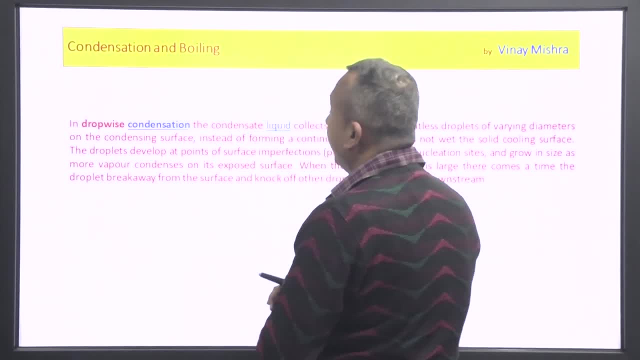 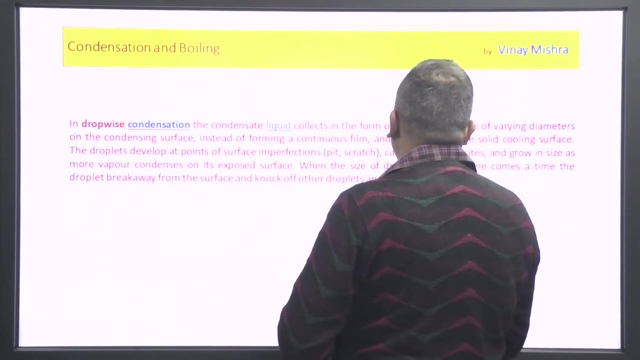 and grow in size as more vapor condensed on its exposed surface. When the size of droplets is large, there comes a time the droplets break away from the surface and knock off other droplets and carries it downstream. If we take the surface again, 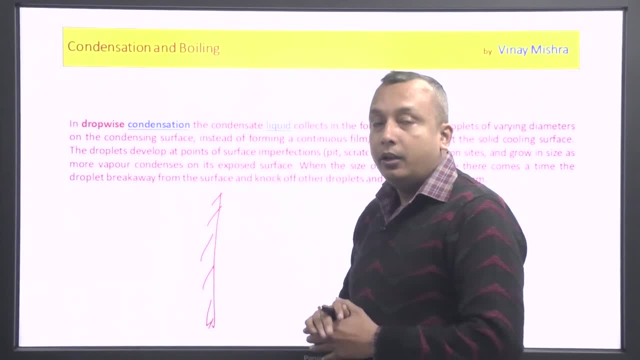 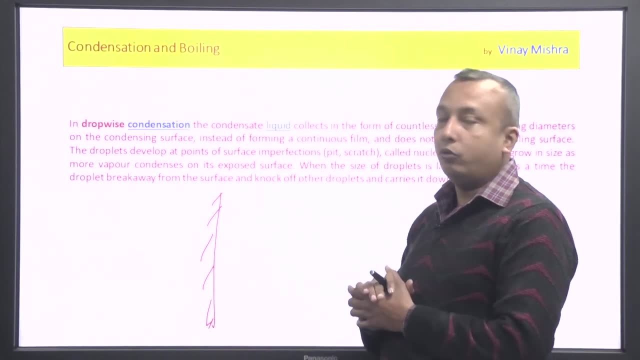 what was happening in the previous case. There film was forming, A layer was forming in the form of film. There condensation was happening. Now, here there is vapor. Let us assume it is about 100 degree centigrade. 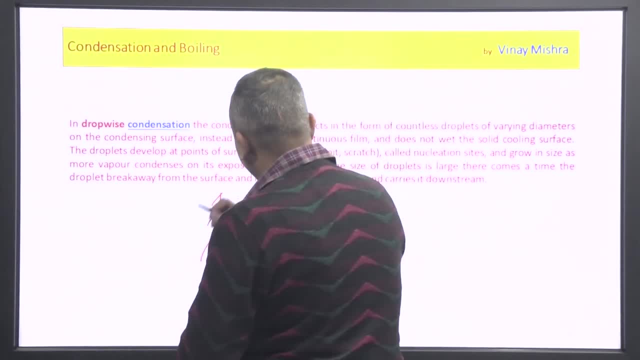 Here there is vapor at about 100 degree centigrade. As soon as its temperature comes in contact with it, its temperature is less than the saturation temperature. The condensation will start Now, due to the start of condensation here. 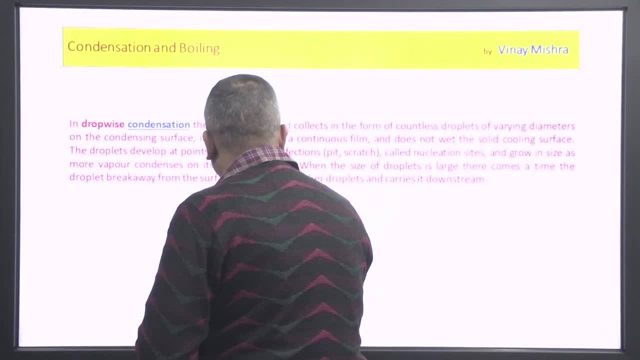 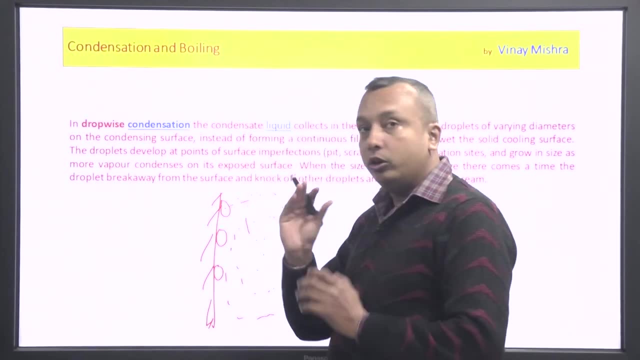 the molecules come in the form of droplets. That is, the vapor. molecules will come in these droplets. These droplets will gradually grow, That is, its concentration will increase. That is, the vapor will not be able to wet the surface uniformly. 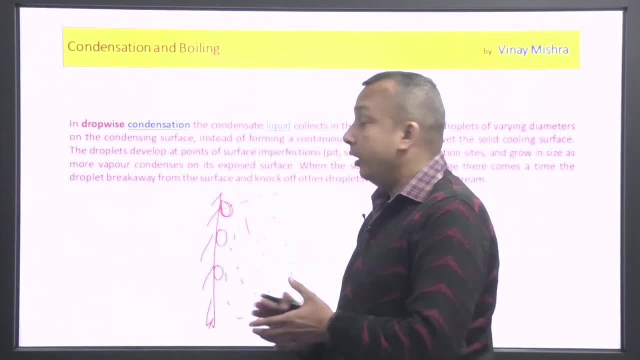 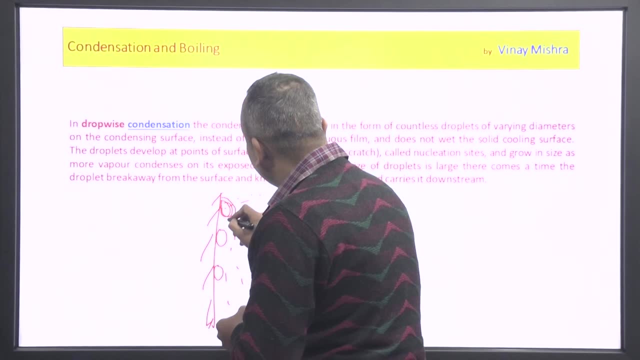 That is, it will not be fully exposed. That is, it will not be fully exposed to water. And there will be some areas where the size of the droplets will keep increasing. As soon as its size increases, the condensation will keep happening. 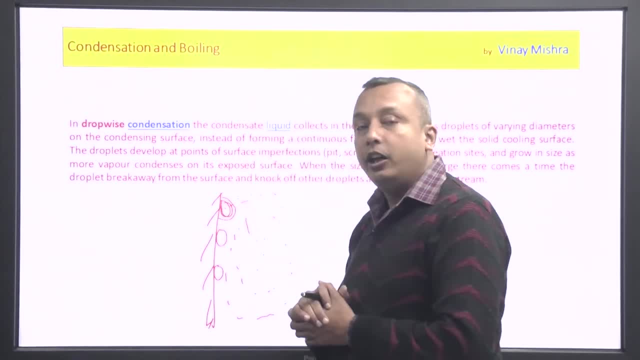 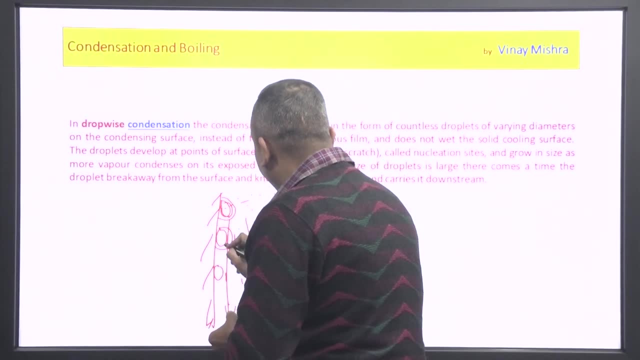 After a certain point, when its size increases by a certain limit, then, due to gravity, it will drop down. If we talk about this drop, then it will also drop down. If we talk about this drop, then it will also drop down. 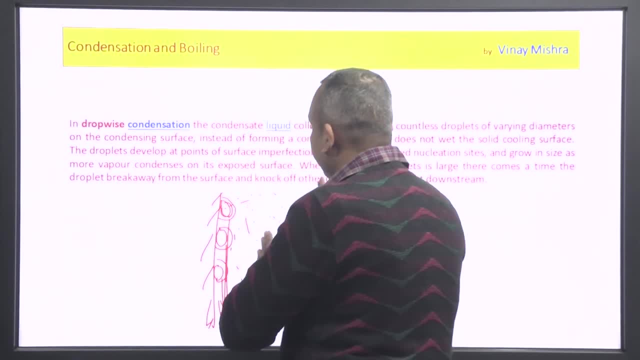 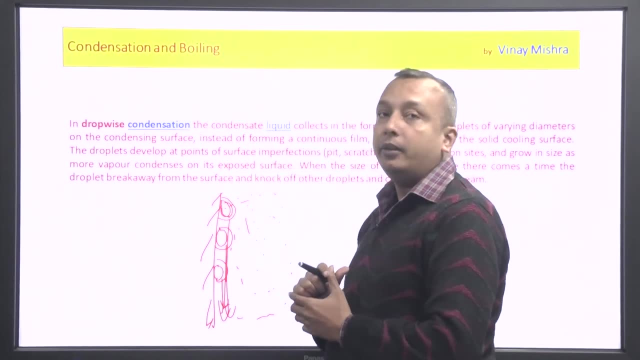 Now what will happen? Now this space is empty Again. here a different molecule of vapor will come. Condensation will happen again. Droplets will be formed. The size of the droplets will increase As the size increases. 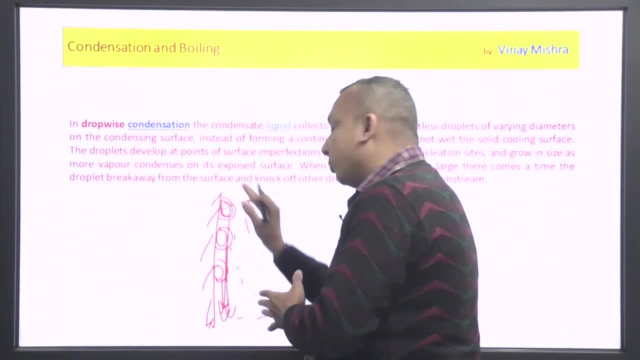 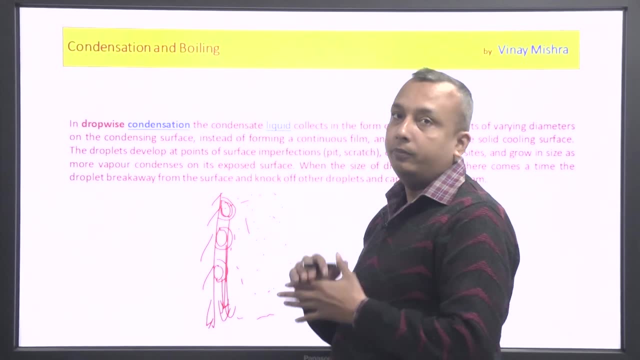 the drop will come down again, That is, that space will be empty again. In this way, the process will keep on increasing. And here the condensation process will keep on going. And here we see that when the condensation will happen in this way, 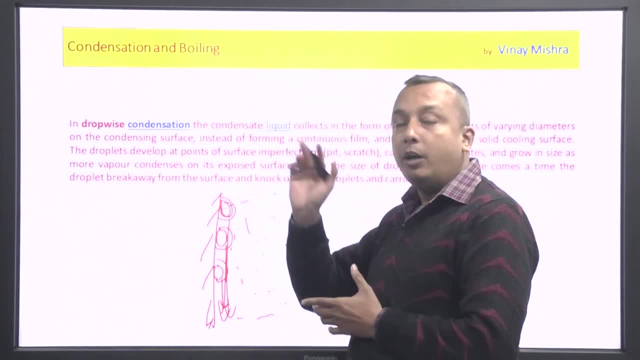 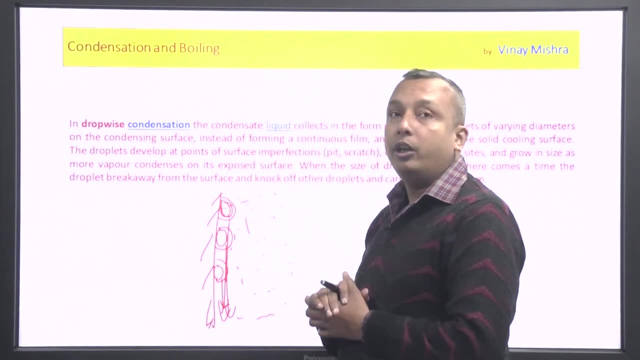 then what will happen Here? the rate of condensation is constant. It was changing there. It was decreasing there because the formation of the film was happening there. Here there is no formation of the film in any way. A drop is being formed. 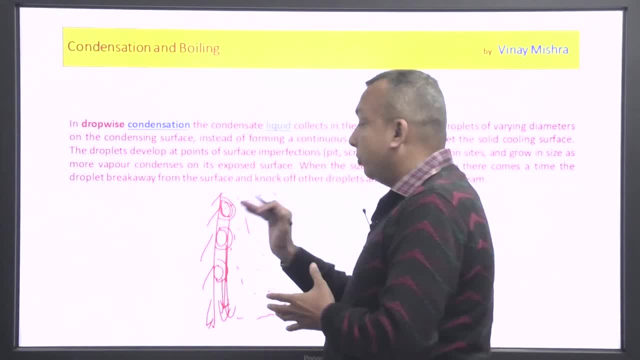 It is coming down again. That space is getting empty. Because of the empty space, because of the empty space there again in that space, other droplets are coming Again. another droplet will be formed, Again. it will come down due to gravity. 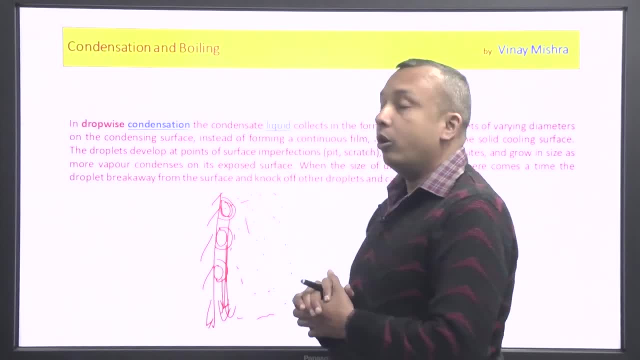 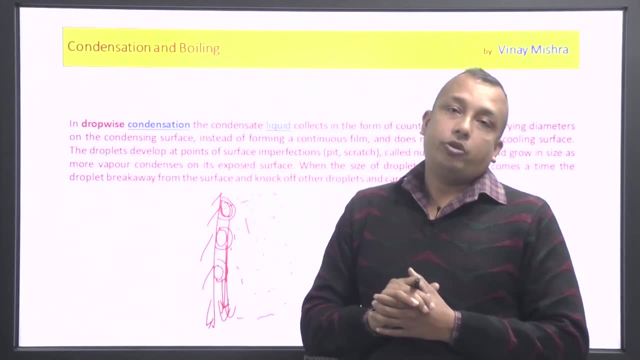 In this way. we see here that here the process of drop-wise condensation will be called drop-wise condensation And here the rate of condensation will be constant. Here the rate of condensation was basically changing and decreasing. Here the heat transformation will not change.